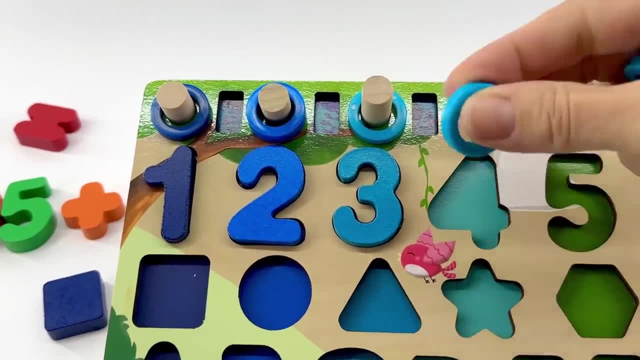 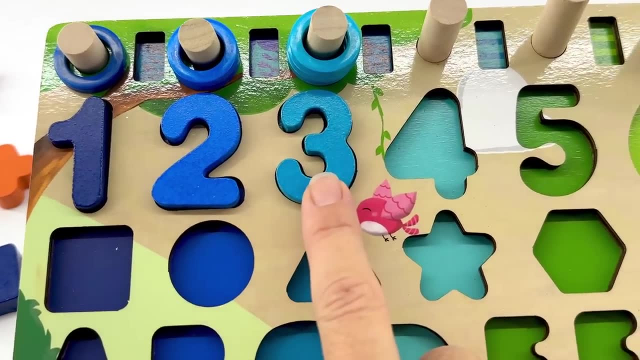 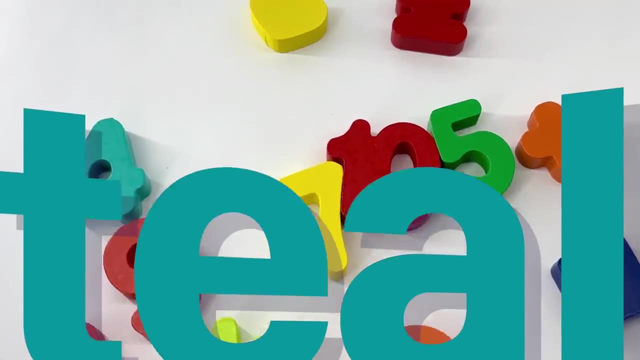 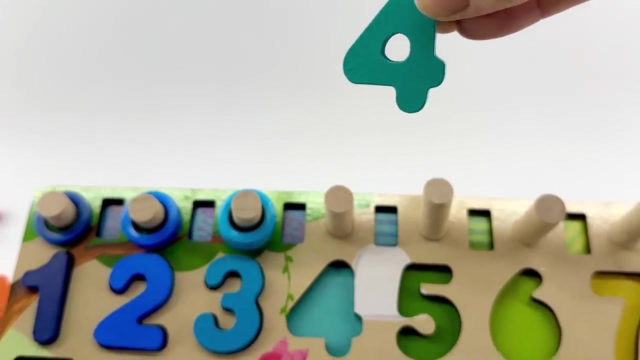 One, Count with me, Two And three. One, two, three. Do you know what number's next? Yes, it's the number four. Do you see a teal number four? Yes, it's right here. You're doing so great Number four, And let's put it in its spot. Now let's count the circles. 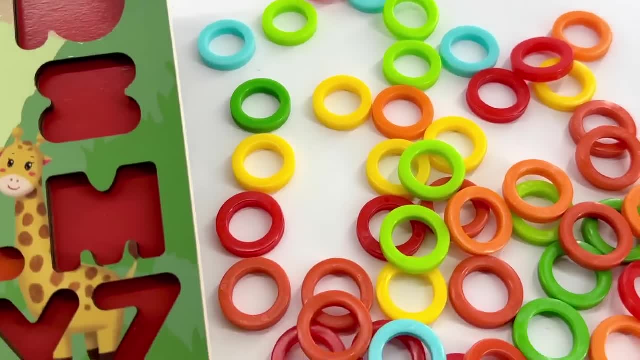 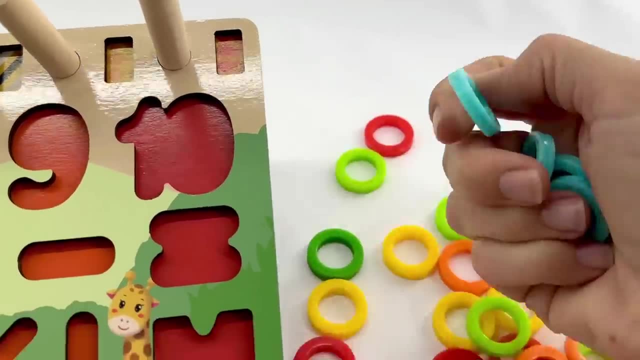 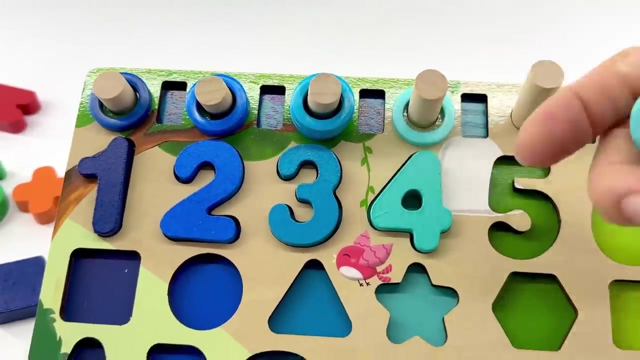 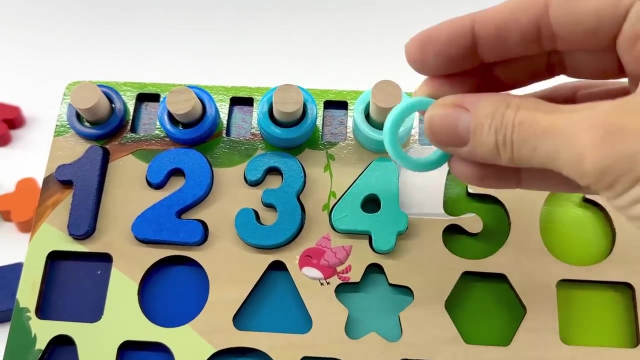 Do you remember that color? teal, I think I see them. Here's one, There's another, one And another. Let's pick them all up and then we're going to count them to make sure we have all the right numbers. Okay, Here we go. Don't forget to count with me: One, Two, Three And four. We made it to number four. Hey, this is a different color. 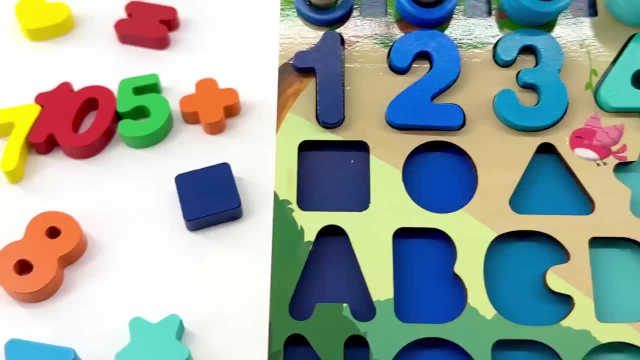 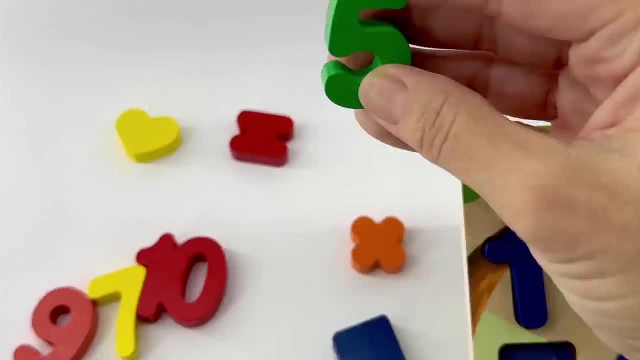 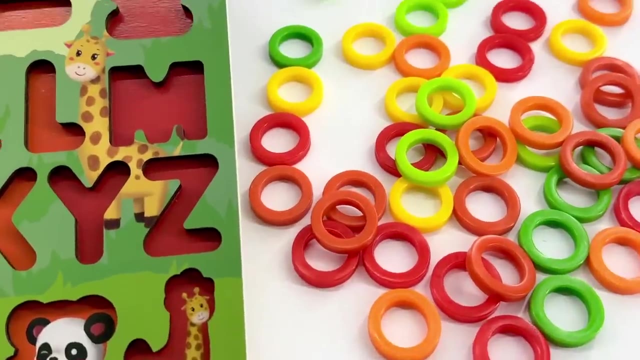 is green and that's the number five. that's a dark green. do you see a dark green number five? yes, I do see it. it's right here: dark green number five. okay, put it right there and you know what to do next. we need to find five dark green. 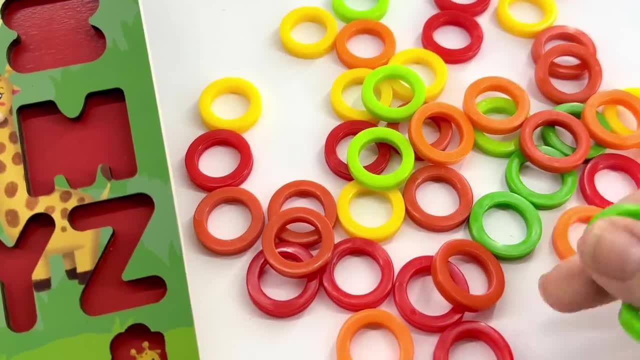 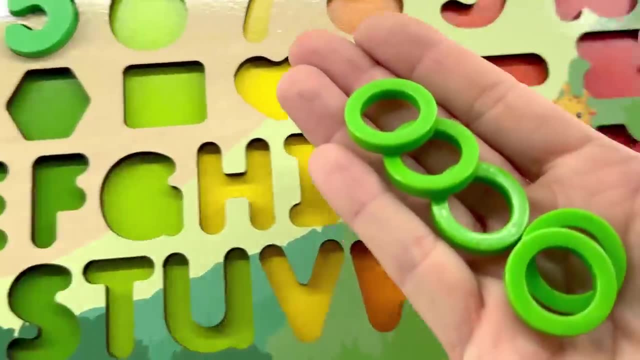 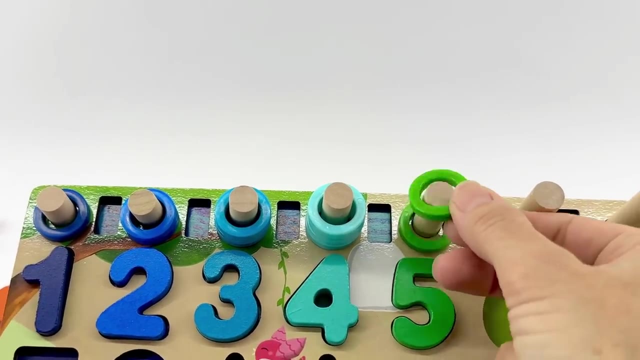 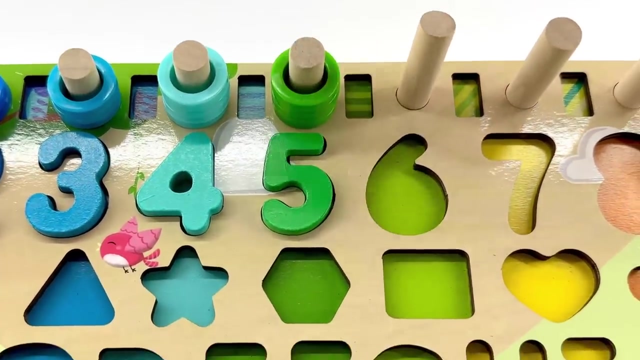 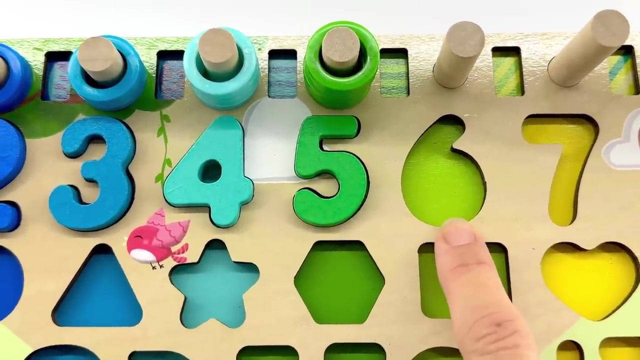 circles. here's one, there's another one. boy, there's a lot of circles to pick up. now hold them all in my hand. okay, let's count and make sure we have the right amount. count with me one, two, three, four and five. yep, that's number five. next we have the number six. this is a lighter green do. 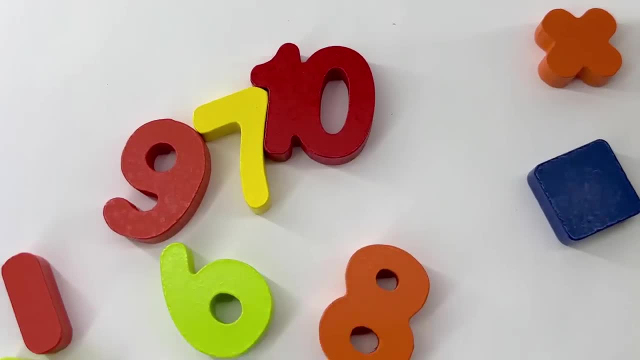 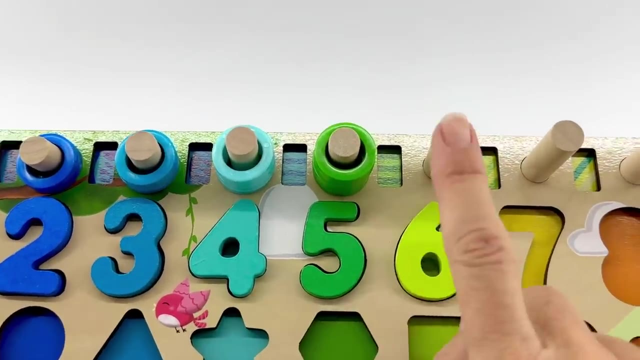 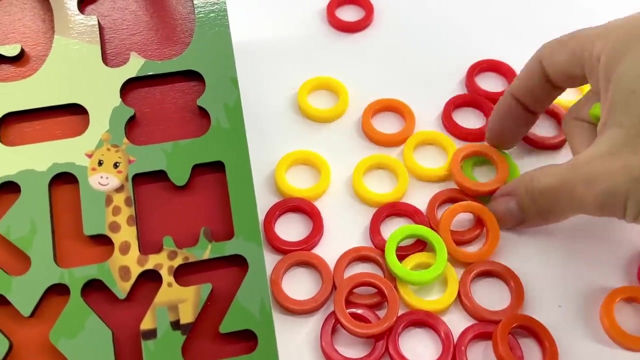 you see a number six. that's light green. yes, I do see a light green. yes, it's back here. you got it, number six, light green. okay, put that there and next for our circles. but let's make sure we have all six. let's pick them up. help me find them. oh, one was hiding under the orange, okay, 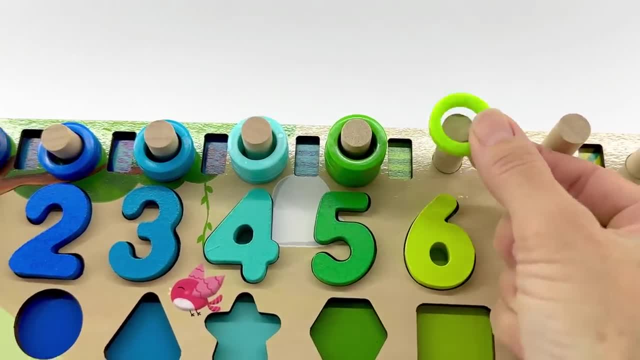 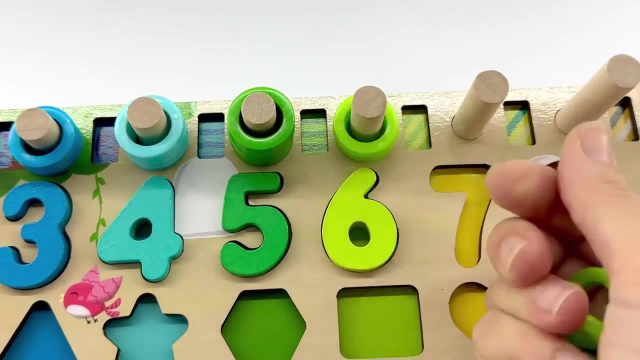 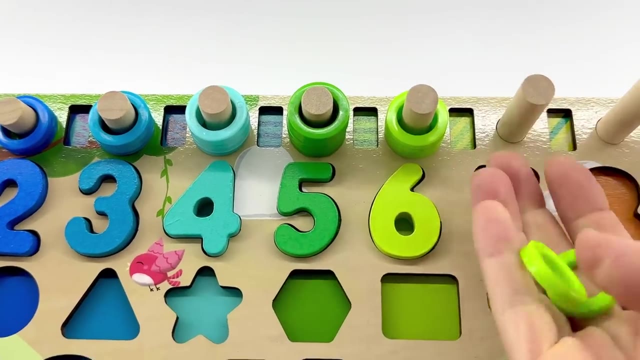 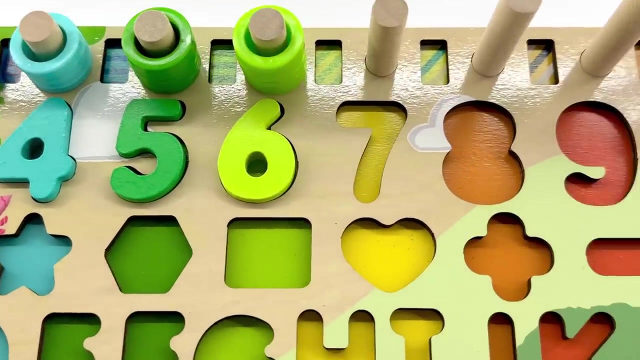 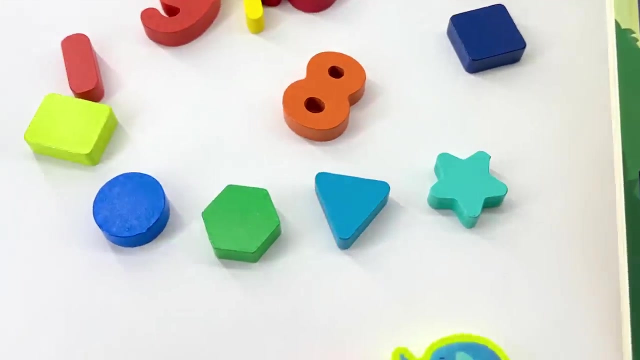 count out loud with me. here we go: one, two, three, four- oh, I gotta get it in my hand- four, five and six. you're doing great, hey, what color is that? that's the color yellow, and that's the number seven, and there's only one yellow number seven. here it is. we'll put it right there now, will you? 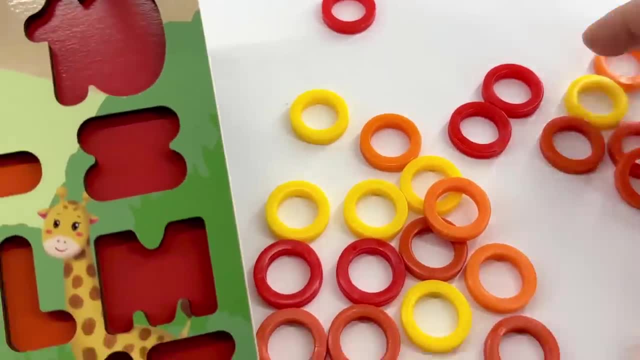 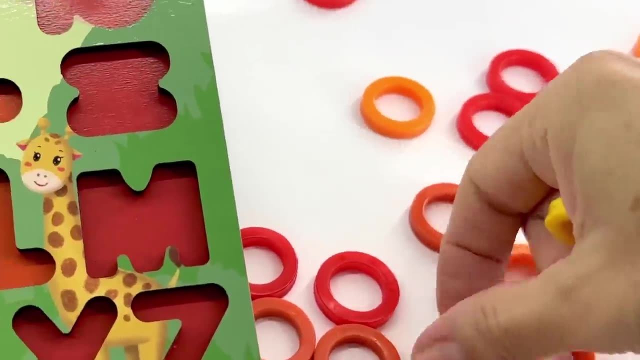 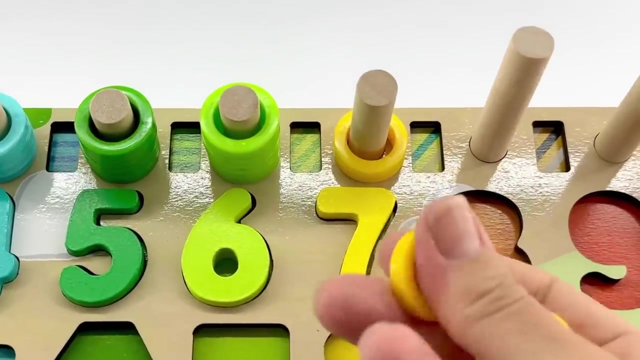 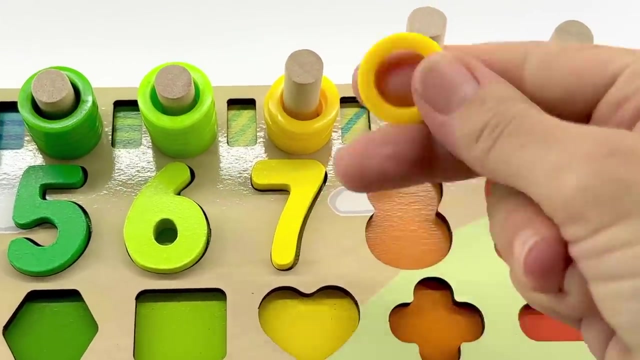 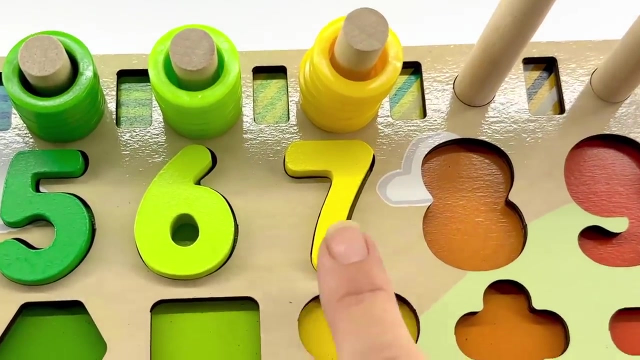 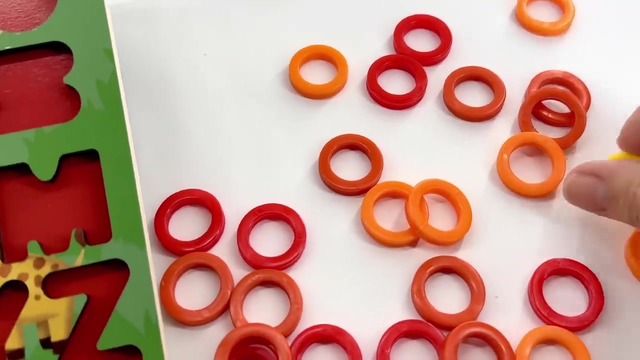 help me count to seven with our yellow circles. okay, let's gather them up. and here we go. and here we go. one, two, three, four, five, six. oh, that's just six. we're missing one. where did it go, oh, oh wait, it's hiding underneath the orange one. there we go. number seven we're. 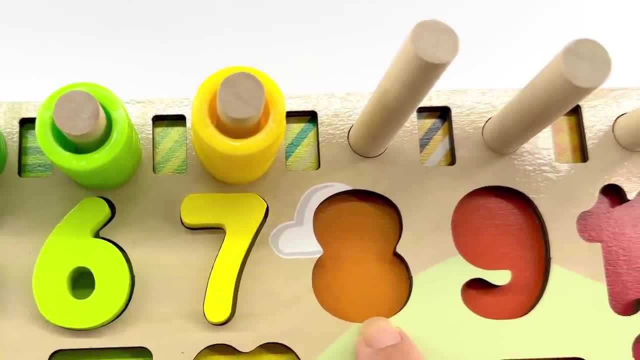 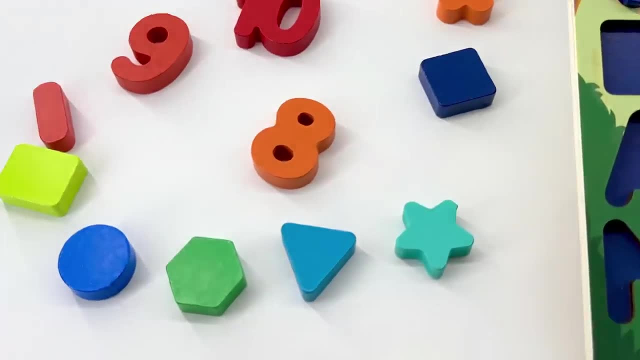 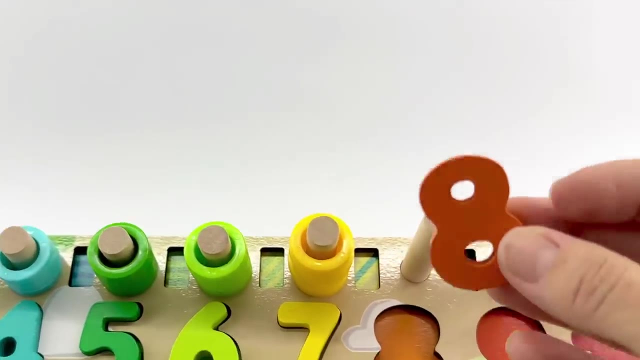 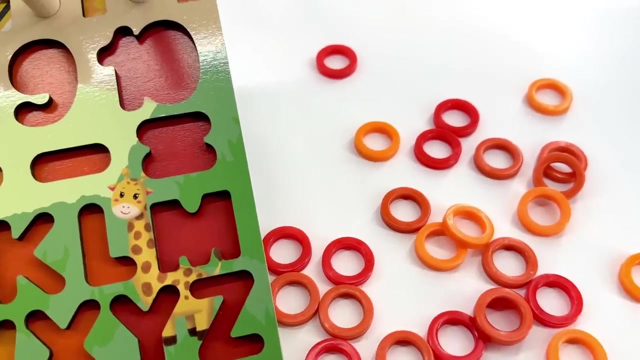 almost there. do you know what number this is? it looks like two circles. it's the number eight, and this one is orange. do you see a number eight? that's orange. right here, it is the number eight. and now let's count. well, this one might be kind of hard to see. we have some light orange. why don't we start with those? okay? 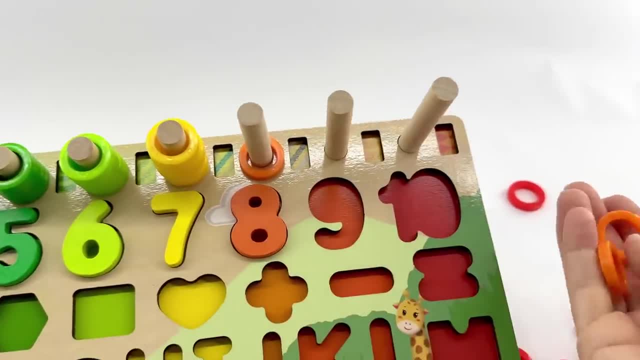 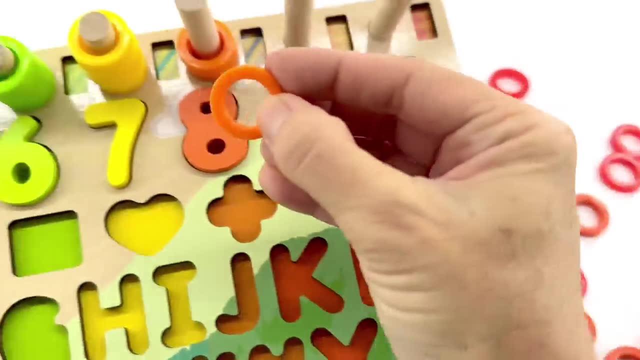 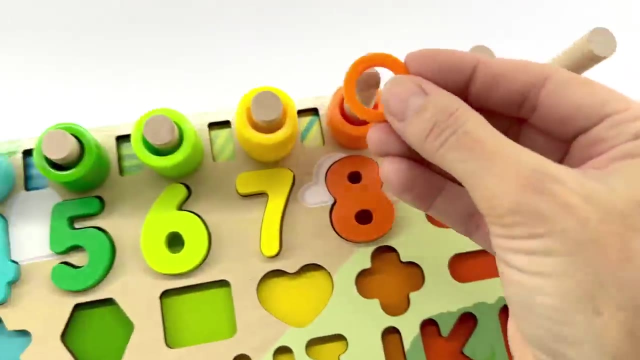 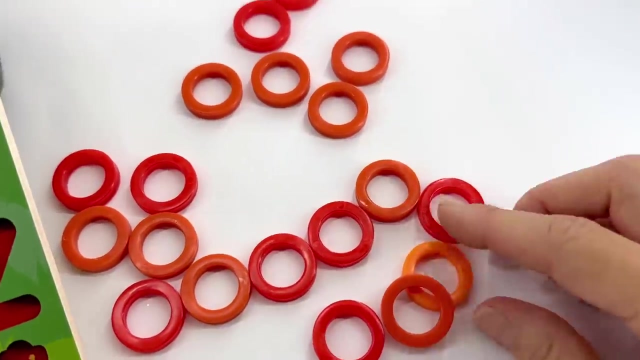 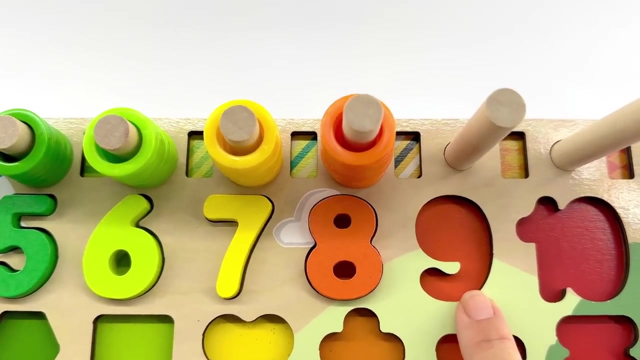 count with me: one, two, three, four, five, six, seven, and there should be one more. yes, here it is eight. that's number eight. now we have number nine. yes, five, number nine, That's a dark orange. And do you see the number nine, dark orange? Right here it is. 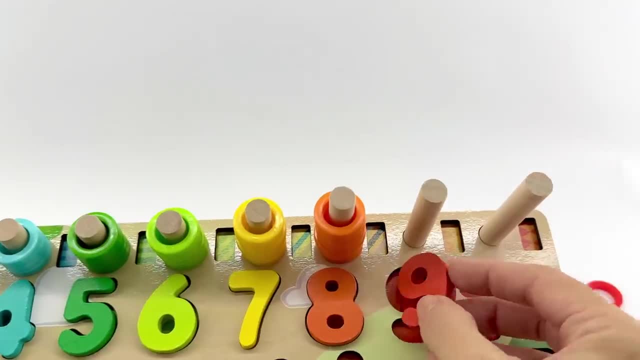 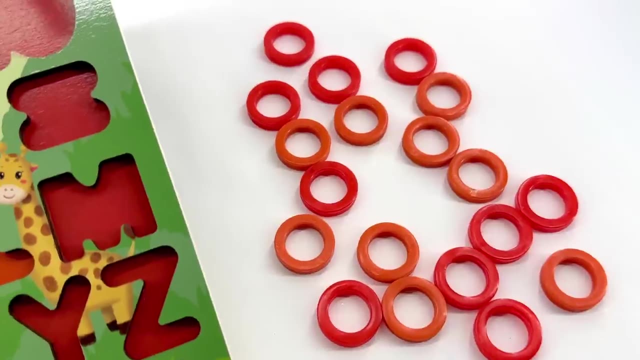 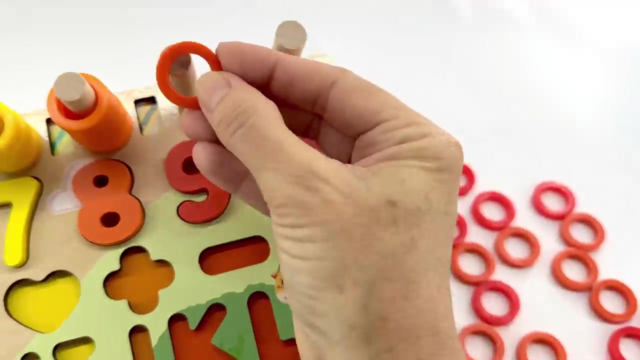 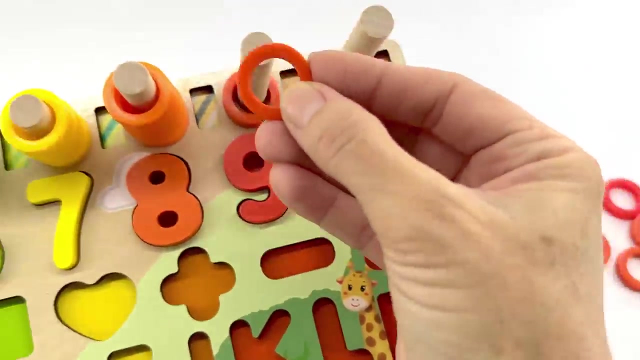 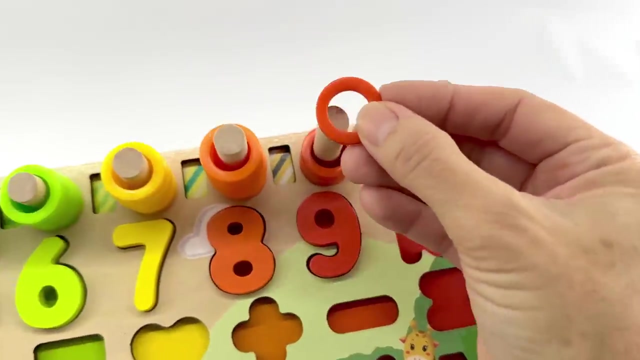 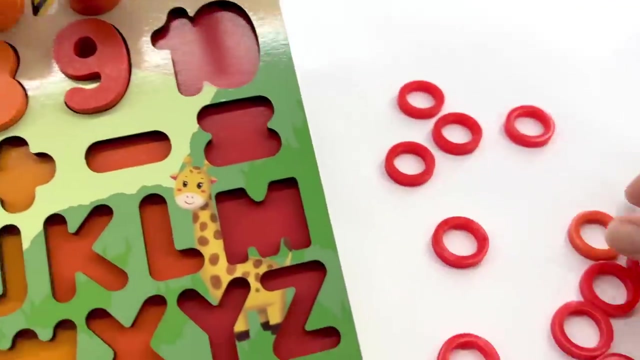 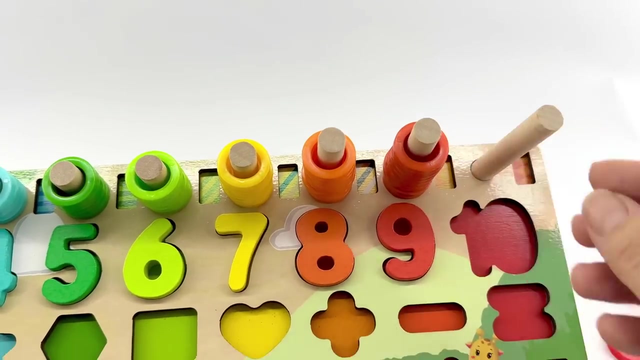 Number nine. Okay, let's put it right here in its spot. Wow, this is really close this color. Some look orange and some look red. Can you help me find all of the orange circles? Okay, here's one, two, three, four, five, six, seven, eight and nine. We did it. I'm so proud of you. 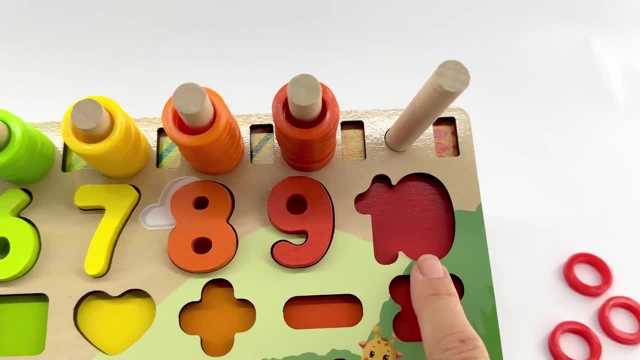 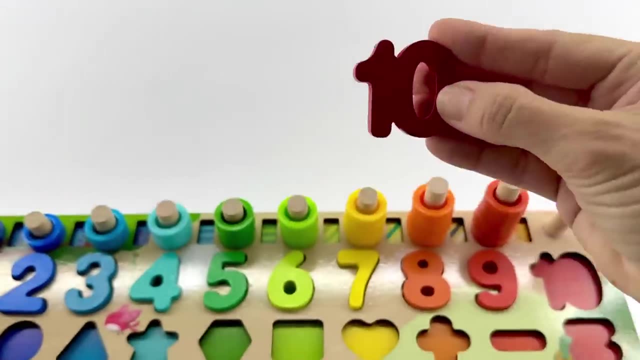 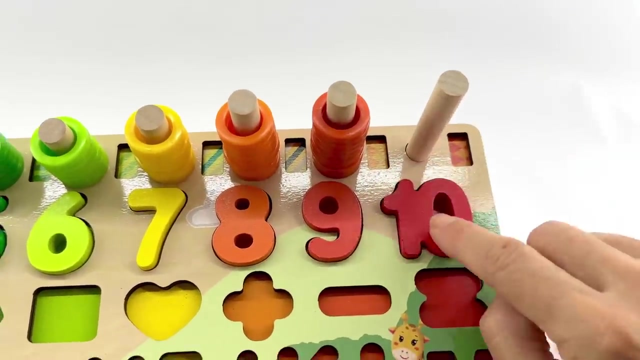 Hey, what's our last number? Last number here, That's the big one, number 10.. And I think you can point out the number 10 to me Right here, it is Number 10.. Let's put it in its spot. Oh no, it fell. Put it in its spot. 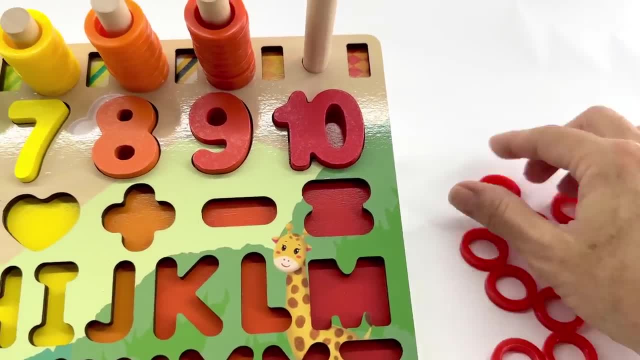 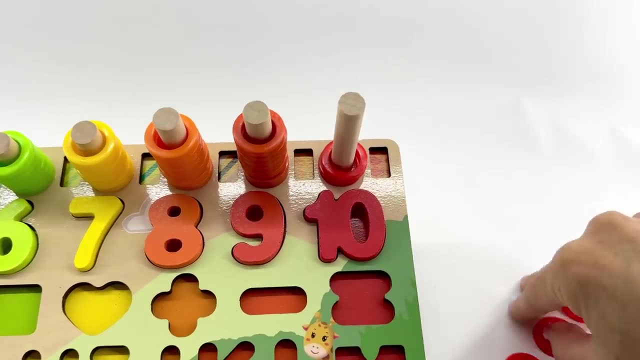 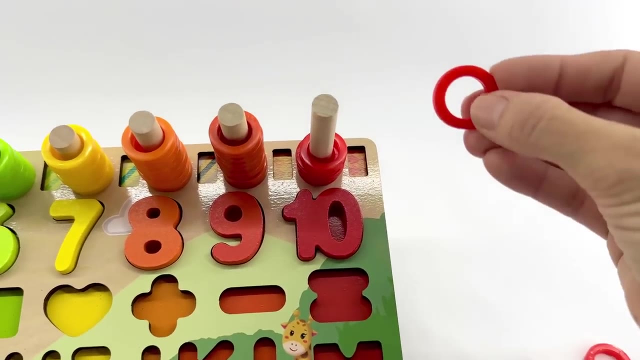 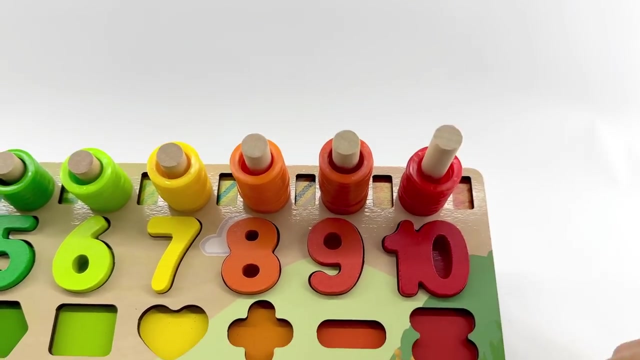 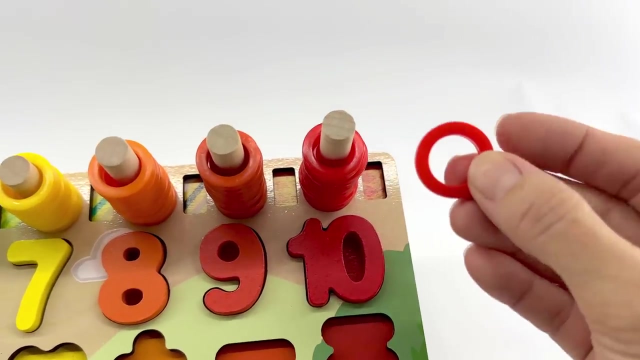 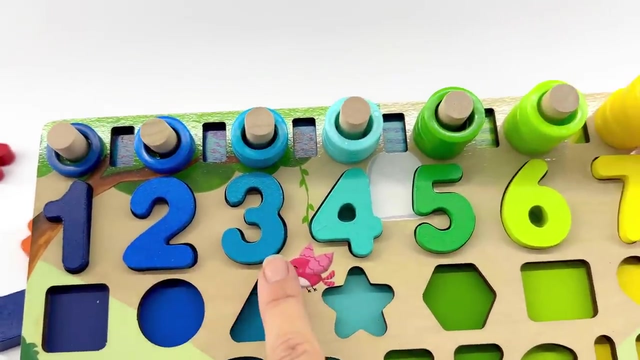 And now you can help me count. These are all the circles we have left. Count with me loud: One, two, three, four, five, six, seven, eight, nine and 10.. You did it. Help me count all of them one more time: One, two, three, four, five, six. 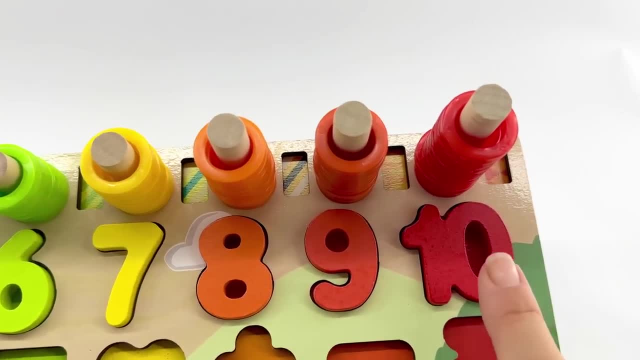 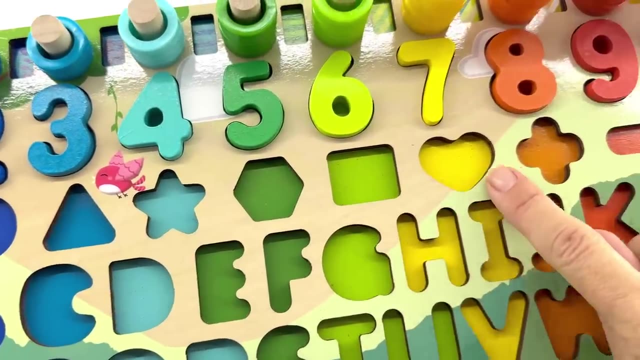 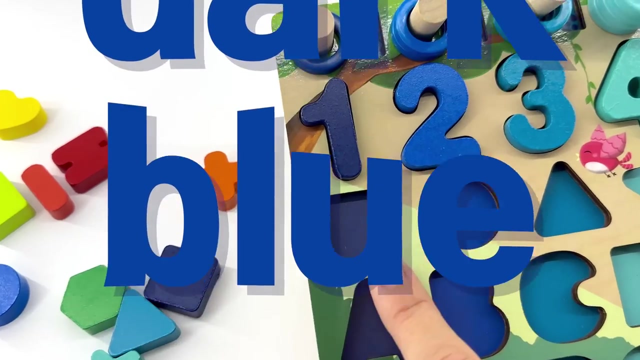 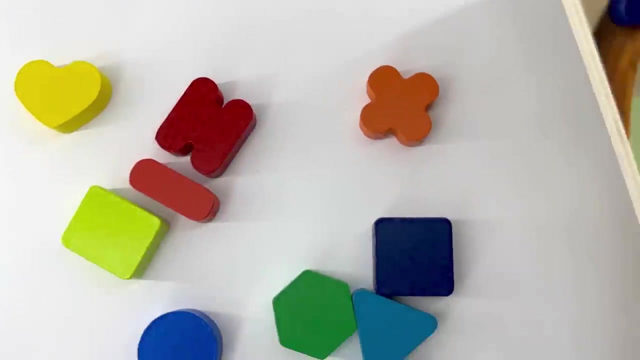 seven, eight, nine and 10.. Right, What are all of these other shapes we are missing on the board? Will you help me fill them in? We practiced our colors, so I think this should be easy. Let's start with dark blue. Do you know what shape that is? Yes, it's a square. And looking at these shapes here, do you see a dark blue Right Here it is Dark blue square. 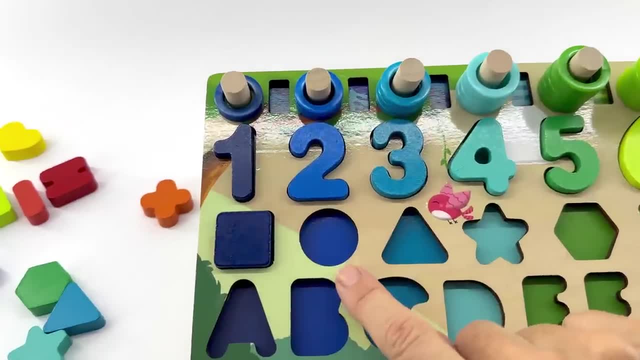 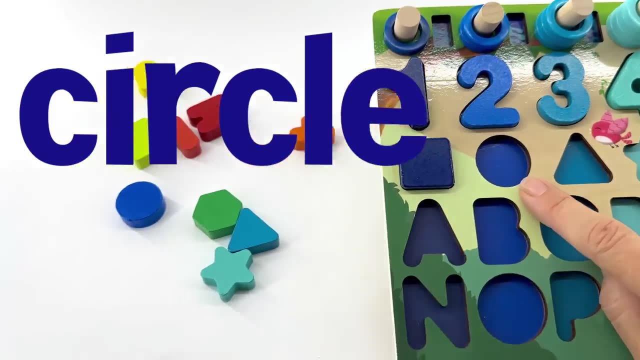 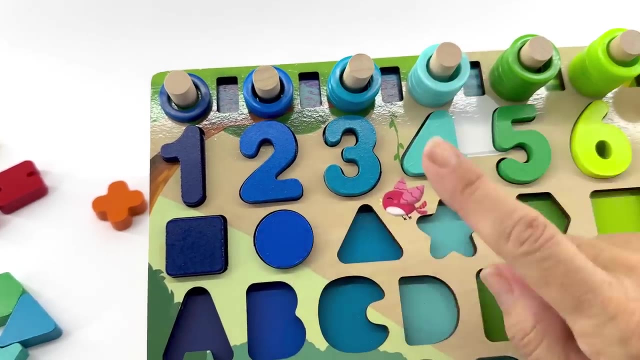 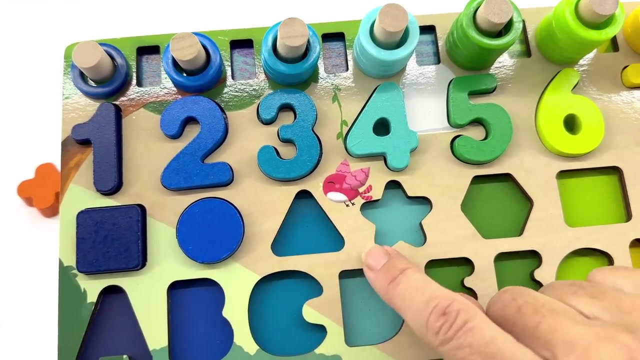 And here we have blue. What is that? Think real hard. Right, It's a circle. Can you point to the blue circle? Good job, Blue circle. Here is a blue. what is this? It has three corners and three sides of equal length. Right, it's a triangle. Can you point to the triangle? 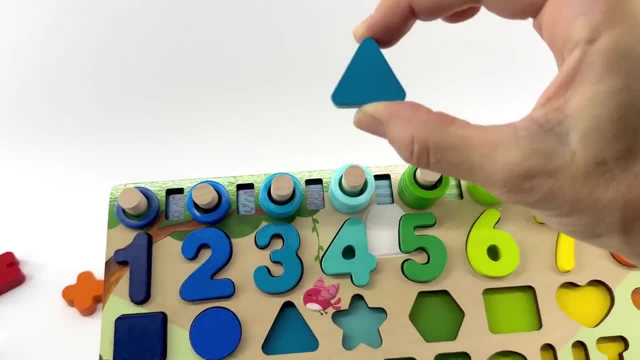 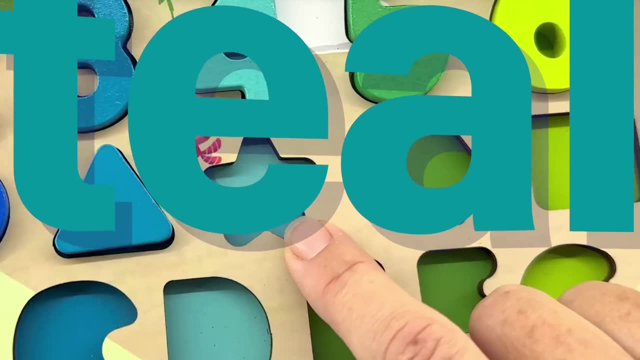 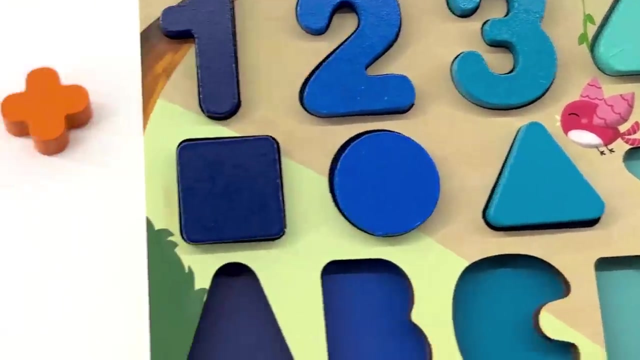 Yes, you did it. Here it is Blue triangle. Look at all of these different shades of blue. Here's our teal. Teal is sort of like blue, but what shape is that? When you look up at the sky real high, you see it. Right, it's a star. Do you see a teal star? You did great. Here you go. 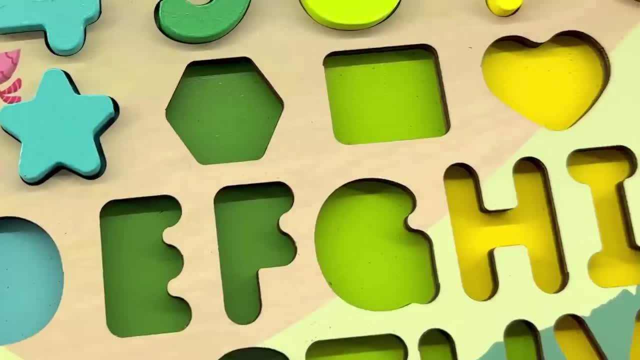 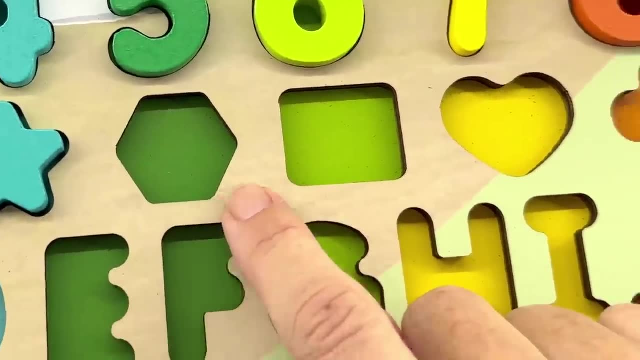 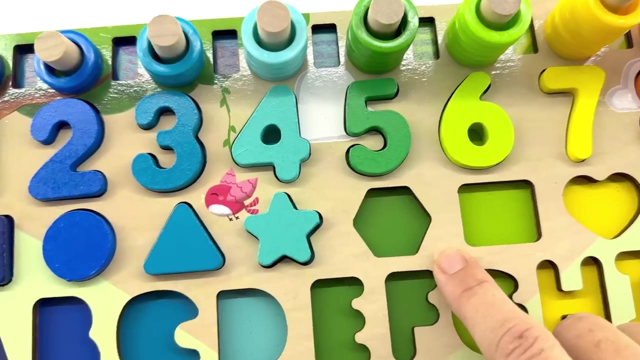 Let's put it right there, Okay, and next we have. what color is this? Right, it's dark green. What shape is that? It's a hexagon: Six sides of equal length and six corners. Now let's find our. 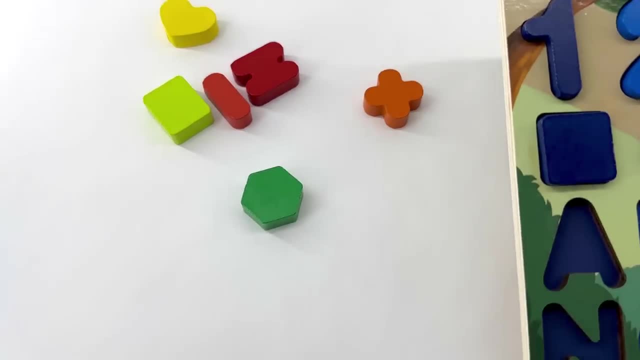 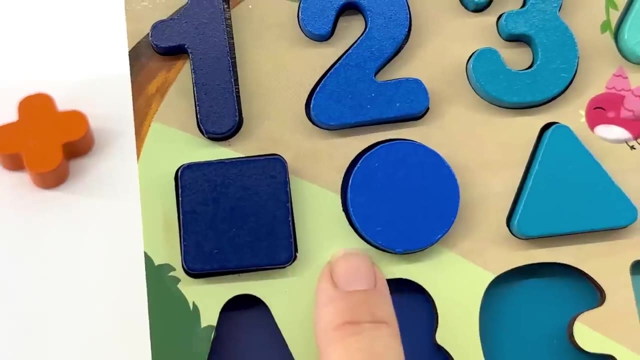 green hexagon, Point to it. Yes, you got it: Green hexagon. What about this? It sort of looks like the square. What about this? It's a square. What about this? It's a square. What about this? It's. 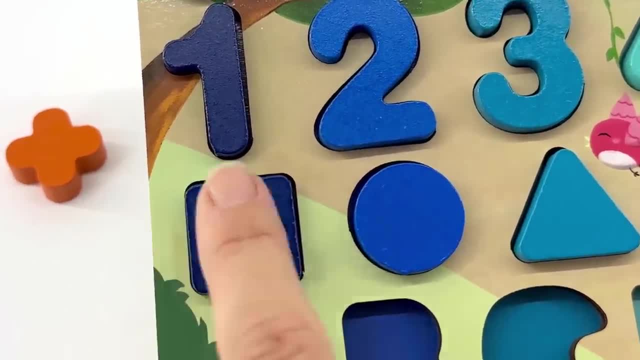 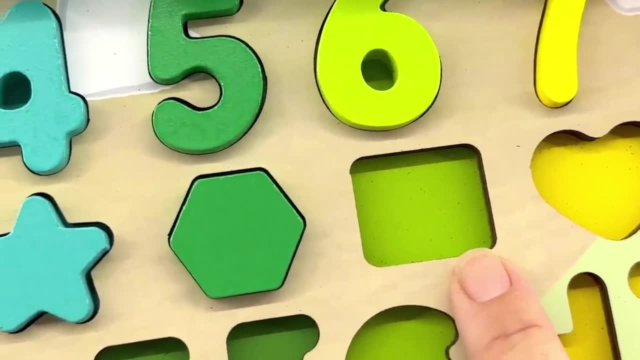 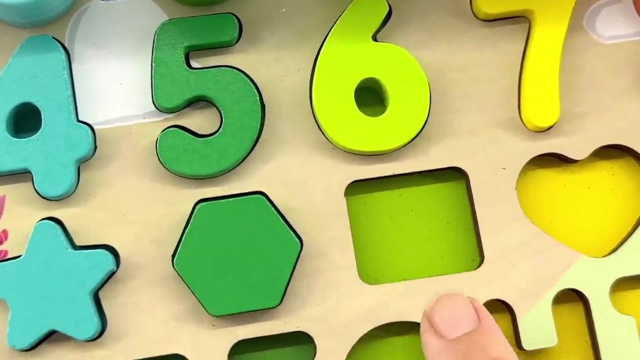 a square. A square has four corners and four sides of equal length. So how is this one different? Hmm, Well, there are four corners: One, two, three, four, But it looks like the sides are different. These are the same size and these are the same size, but different. Yes, it's a. 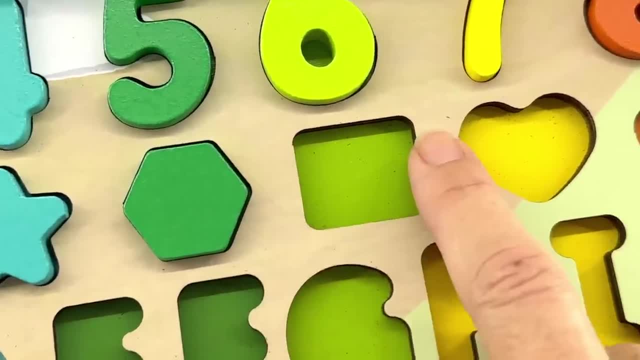 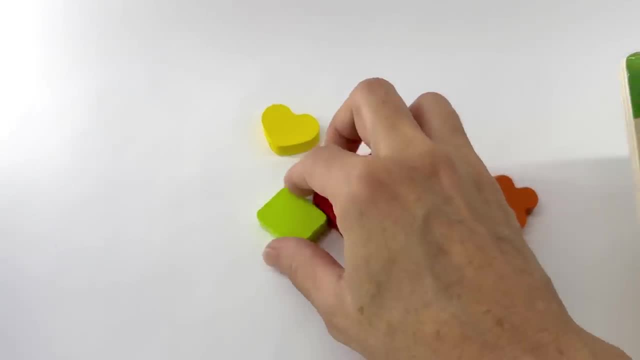 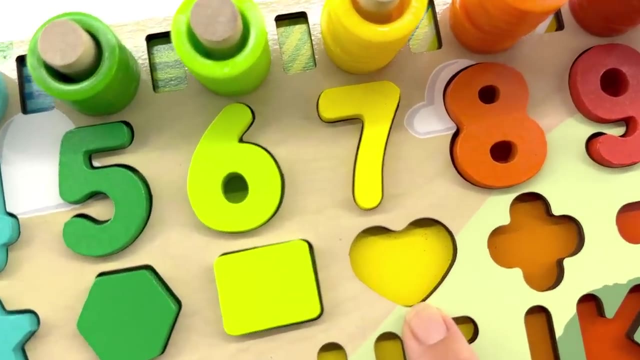 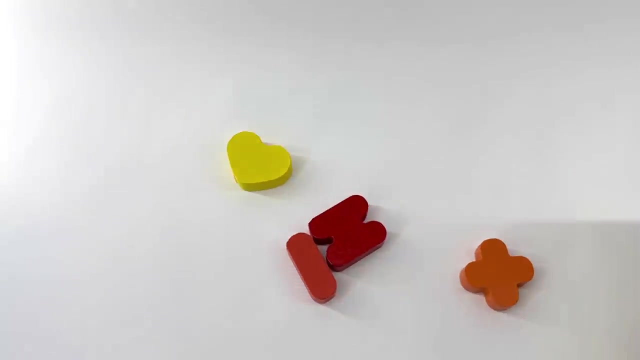 rectangle. A rectangle has two sides of equal length and two sides of different length. Here we go. Can you point to the green rectangle? Yes, here it is Green rectangle And here we have a heart. What color is that? Yes, it's yellow. Okay, let's find the yellow heart. Okay, there's not many. 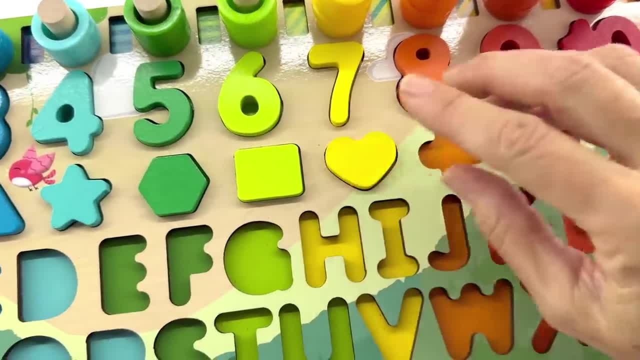 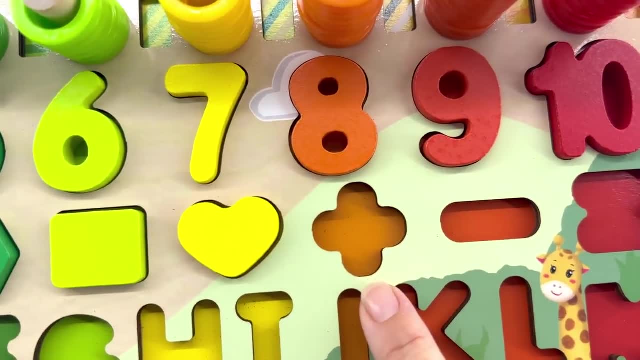 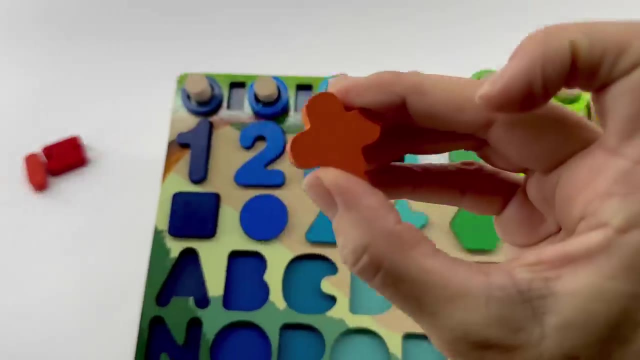 shapes left. You got it Yellow heart. What about this one? It sort of looks like a cross. It's a plus sign and it's orange. Okay, let's find the orange plus sign. Right Here it is. It was almost hiding Orange plus, What about? 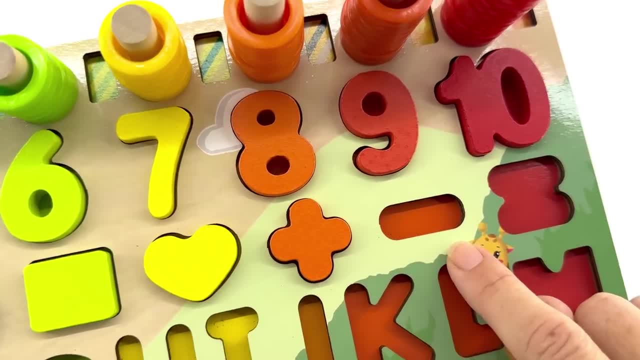 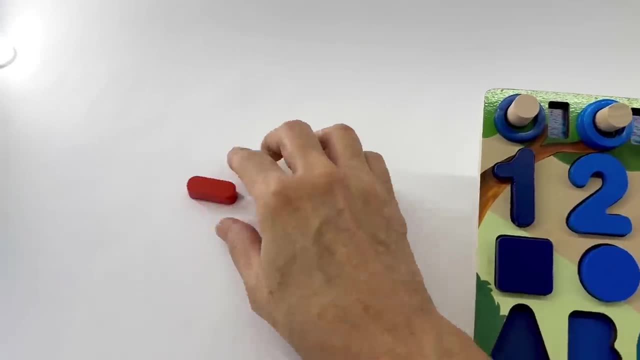 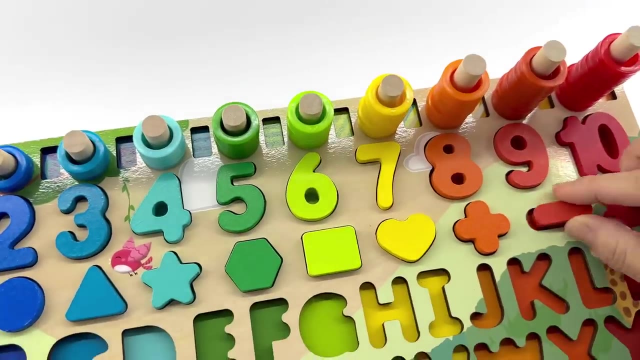 this one, That's orange also, But what symbol is it? It's a subtraction symbol, a minus sign. And do you know which one of these it is Right? It's right here, The orange minus sign, or subtraction. And our last one, right here, This one might. 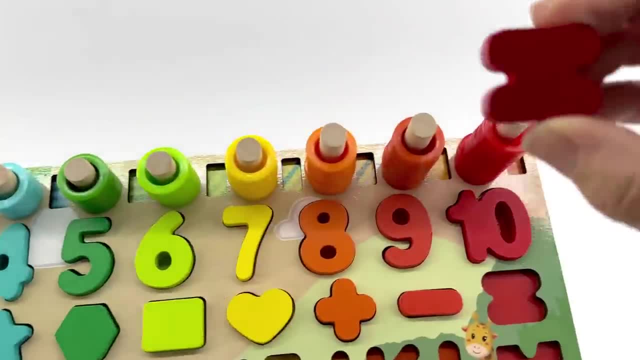 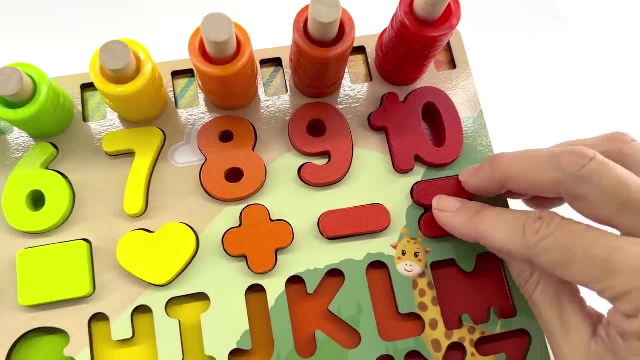 be a hard one. Let me help you out. This one is red and you use it when you are counting in math. It's an equal sign. Put it right there. Good job, I'm having so much fun playing this game. Let's keep going. Why don't we? 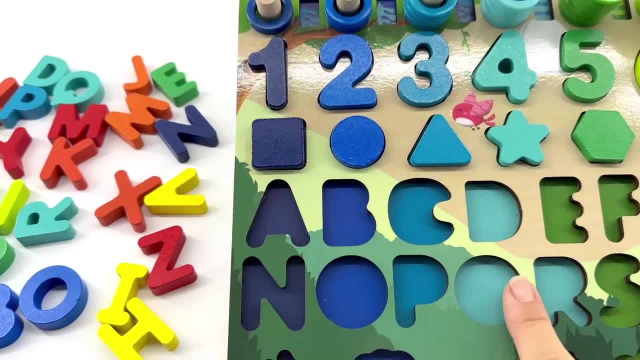 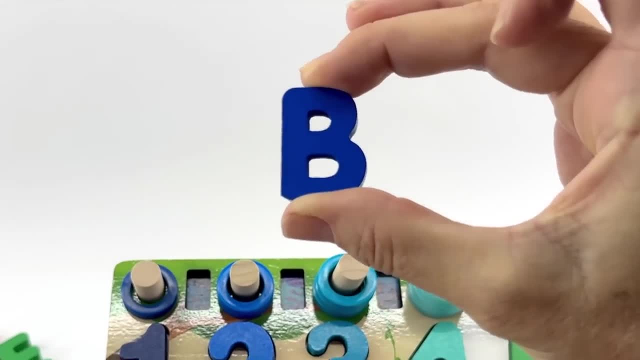 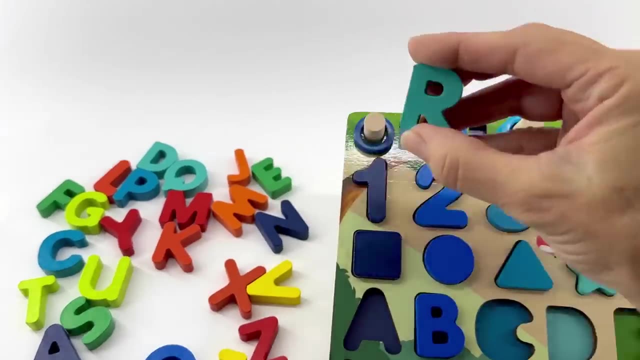 match the alphabet letters with the spot, it goes in and we can put our alphabet together. Hmm, let's start with this one. It's the letter B and it's blue. Hey, B starts with blue. Which one should we do next? How about this one? It's an R. This R is teal. Do you see where the 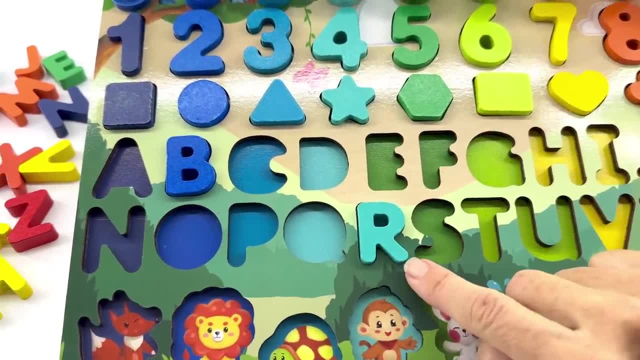 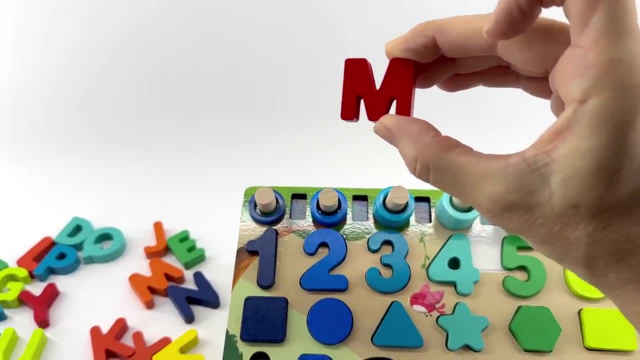 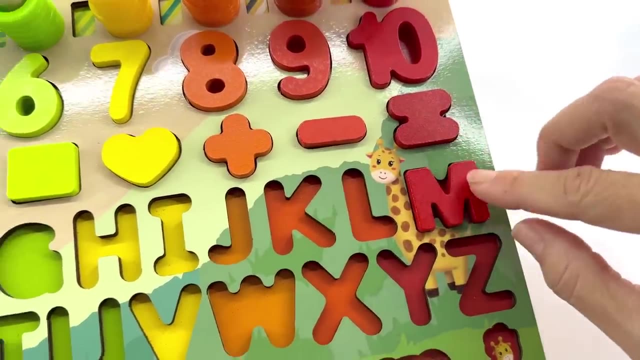 letter R goes Right there Next, why don't we do here? Let's do the letter M. This one is red, The letter M. Do you point? Can you point to where it goes? Yes, there on the end. Now, why don't we do Hey? 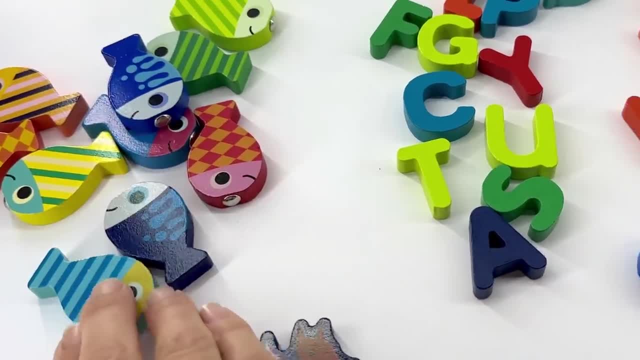 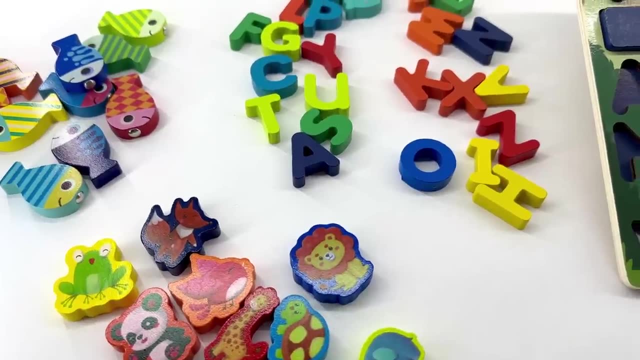 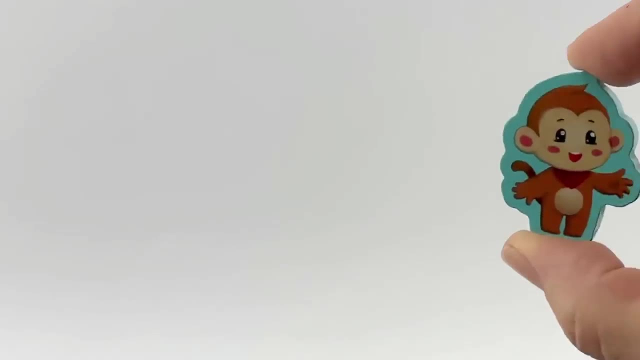 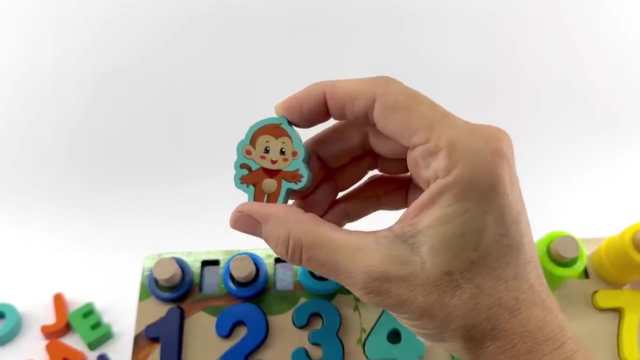 what are those? Oh, these are fish. This is going to be part of a game we do later, But these are animals. Maybe we should try to find an animal that matches one of the letters. Okay, let's play that game. How about what's this? It's a monkey. What letter does monkey start with? Right, the letter M. Hey, we've already placed the letter M. It's right there, Monkey. Now let's find where the monkey 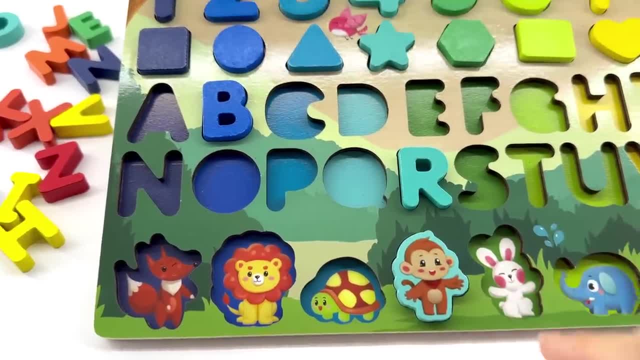 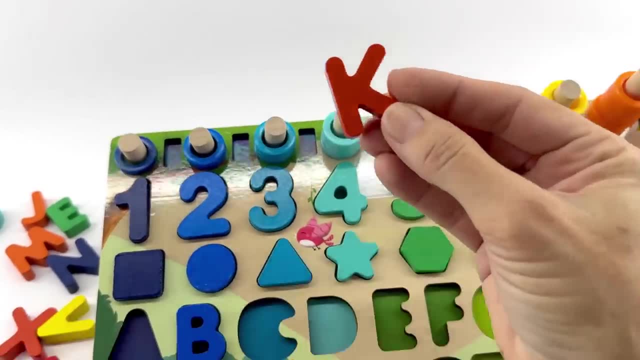 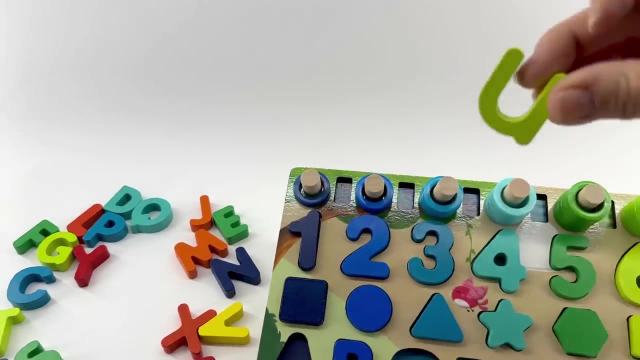 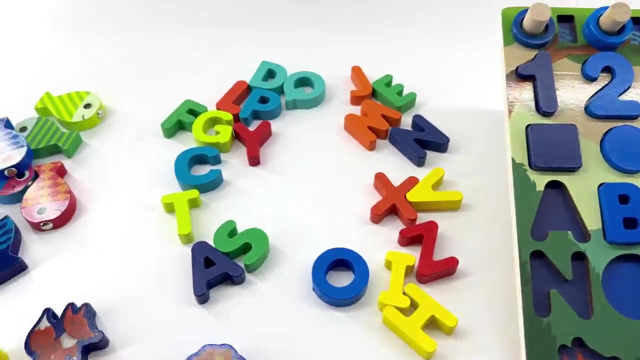 is supposed to go Right there. Why don't we do the letter K next? The letter K is orange, And let's put it in its spot. Next let's do the letter U. This one is green. The letter U goes right there. Now let's do- oh, how about this one? The letter F, And it's green. 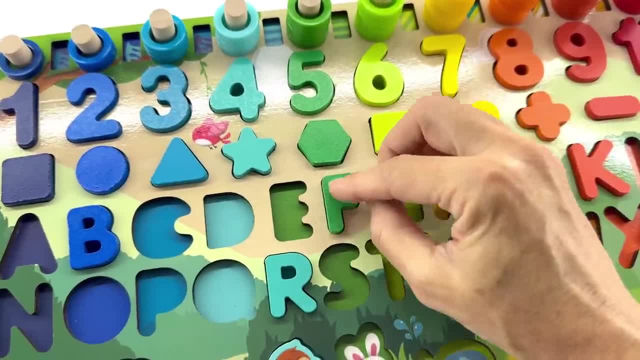 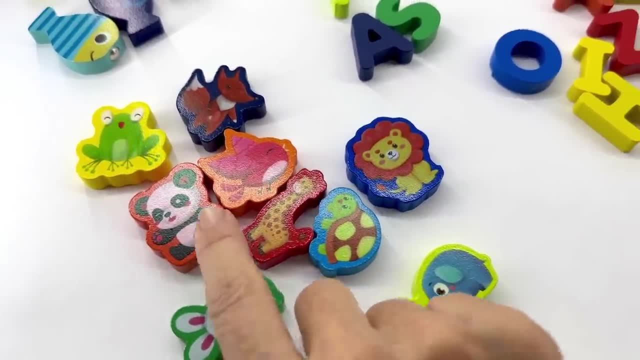 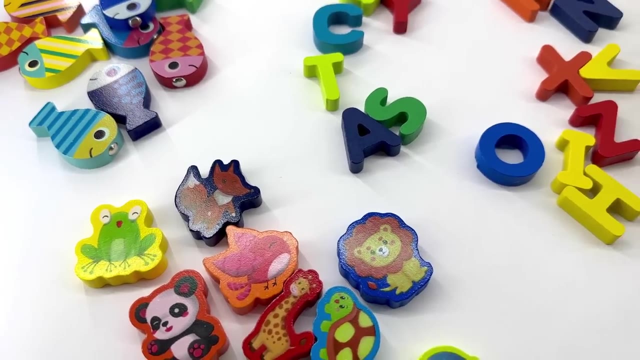 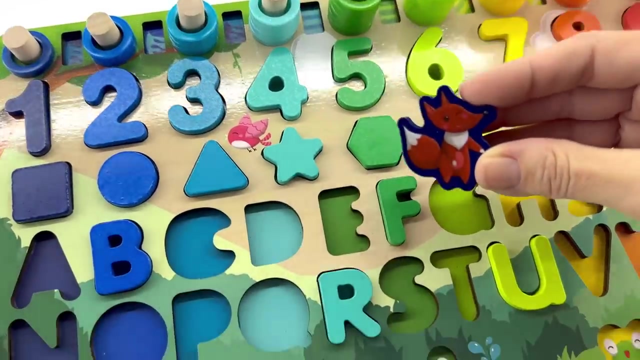 also The letter F. Should we look for another animal that might have one of these letters? Let's see. Well, that's a panda bear, And we haven't done a panda bear yet. A P- What about? Yes, How about a fox? A fox starts with the letter F And we already placed the letter F, So where does the fox go? Right here. 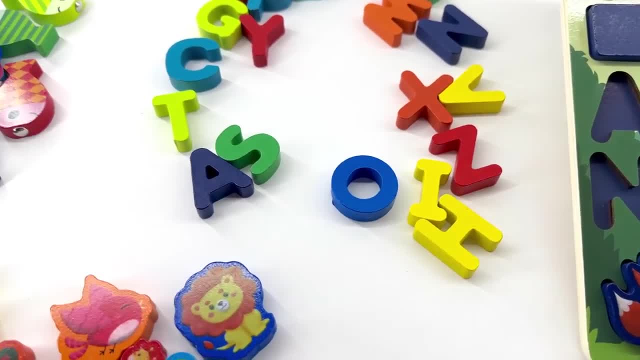 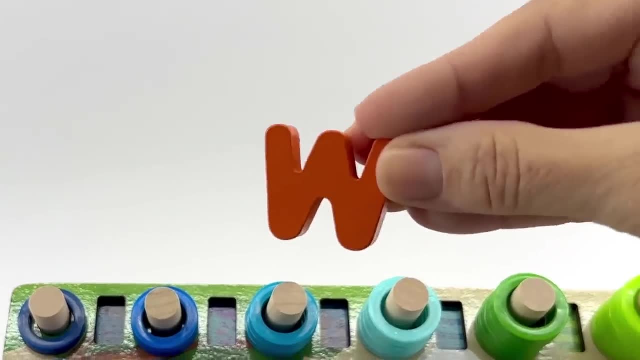 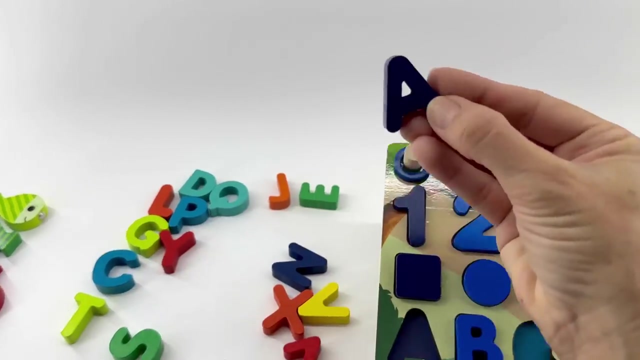 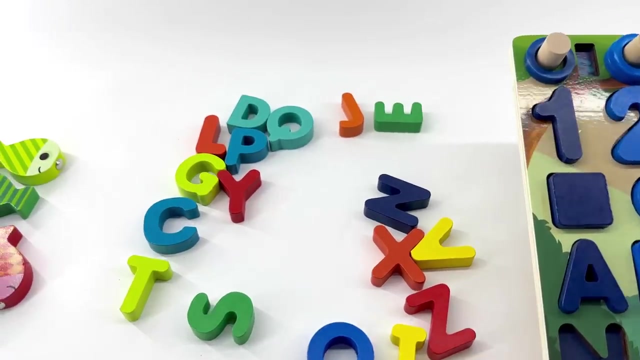 Hmm, Okay, let's go back to the letters. How about the letter W? And this one's orange, Right there. Next, why don't we do the one that starts the beginning of the alphabet, The letter A, And it's dark blue. A. Hmm, How about, here we go, the letter T? It's green. Where is it? 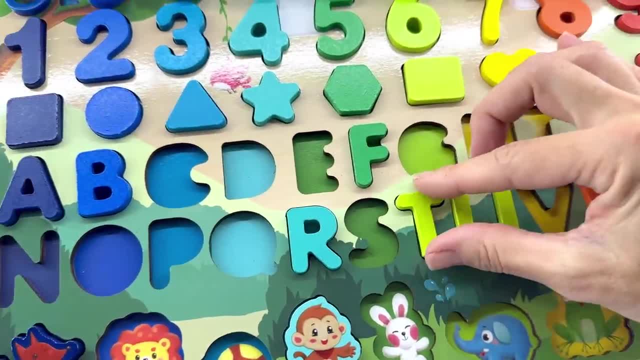 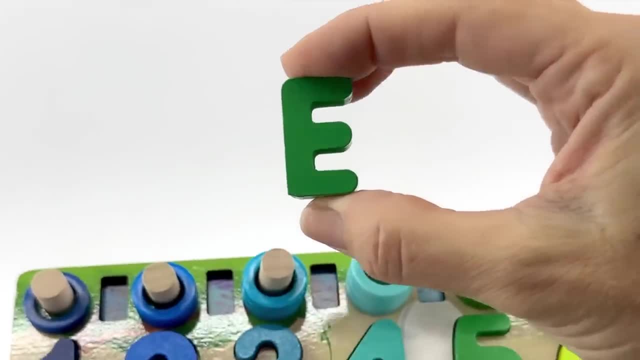 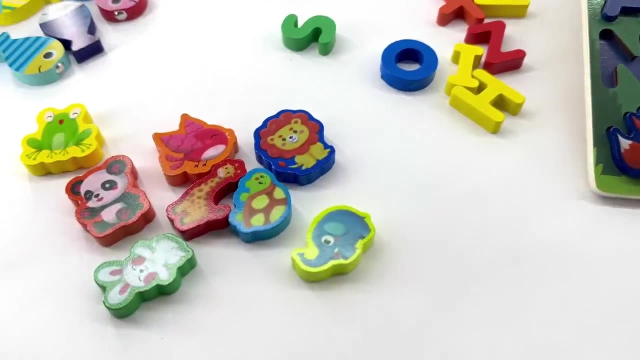 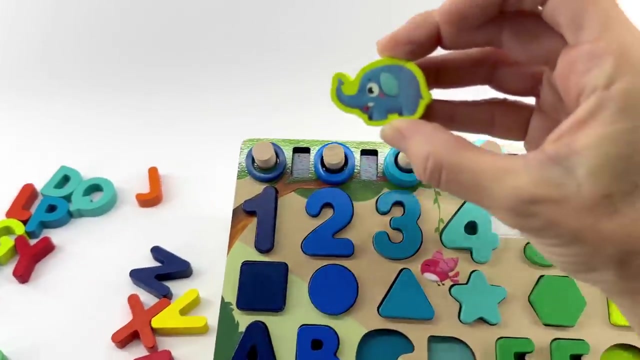 Where does the letter T go? There it is. How about let's do this one The letter E? This one's green. Let's look for another animal that might start with one of these letters. Let's see if there's one that starts with the letter E. E makes an E or E sound. Hey, what about elephant? Elephant starts with the letter E. Let's see if we're right. Yes, we're right. 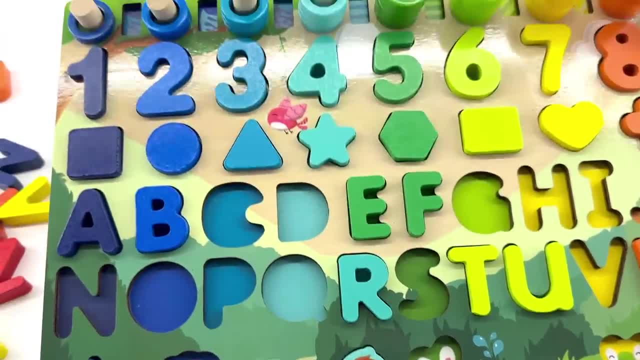 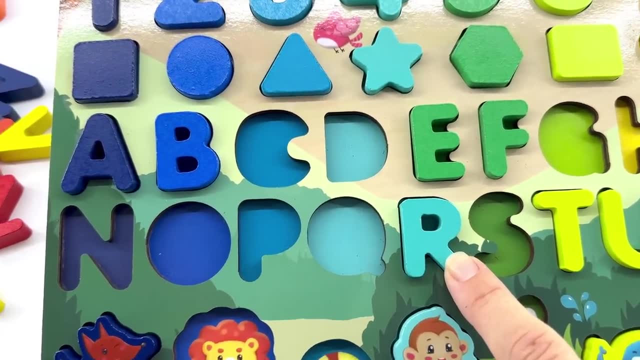 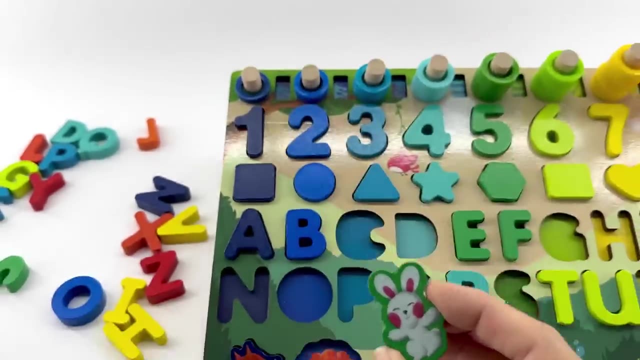 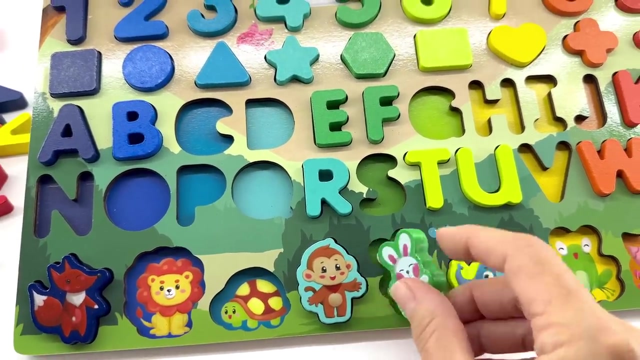 Yes, that's where the elephant goes. You're doing great. Let's try one more. Do you think there's one that starts with an R R makes a R sound Rabbit. Yes, it's a rabbit, And it starts with the letter R. Where does the rabbit go? Right here. Get that to fit. Oh, backwards, There we go. Let's do some more letters. How about the letter K? 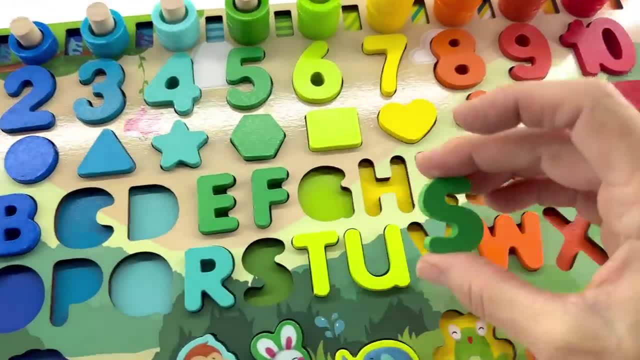 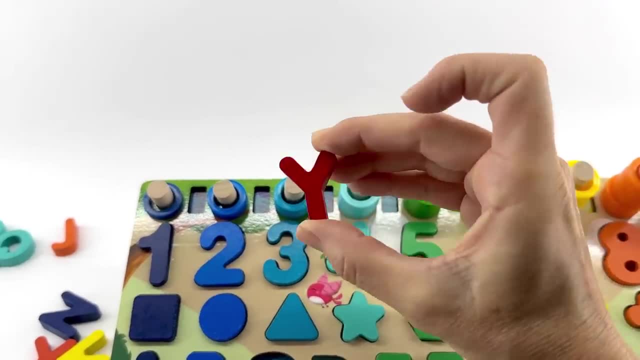 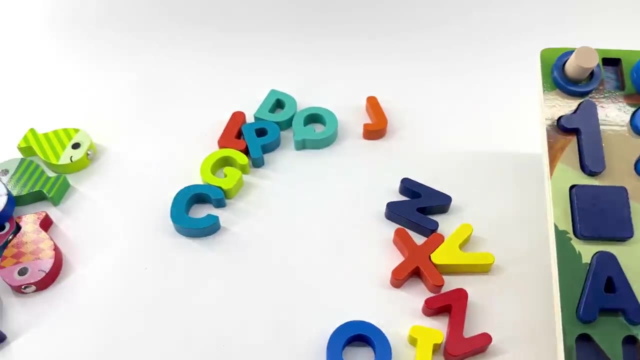 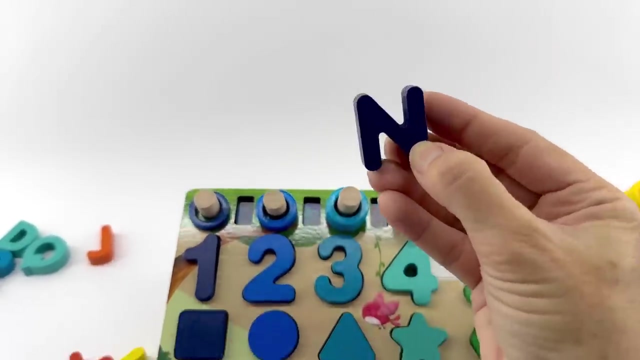 S And it's green. Let's put that in its home. Where does it go There? we go S. Now let's do the letter Y. This one looks like red or dark orange. Let's say it's red. Now let's do how about? how about an N? Make sure we have it right. That's the letter N And it's blue. It goes right here. Do you think there are any more animals? 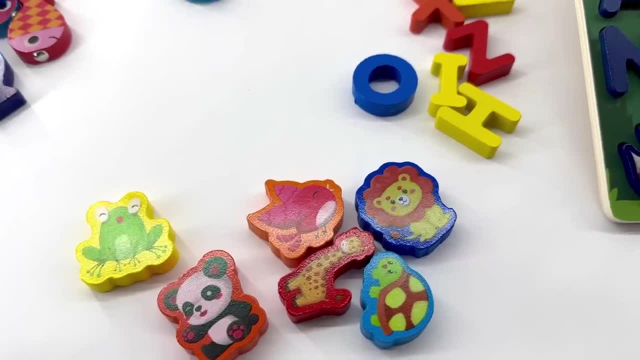 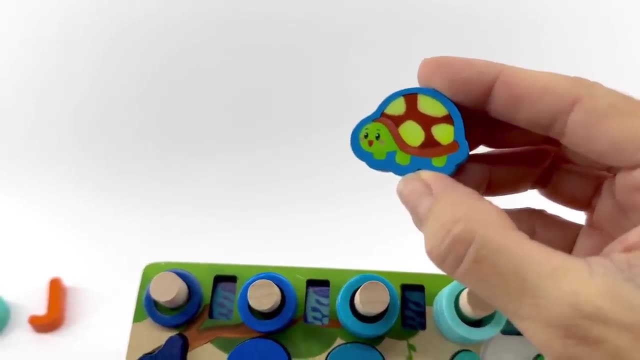 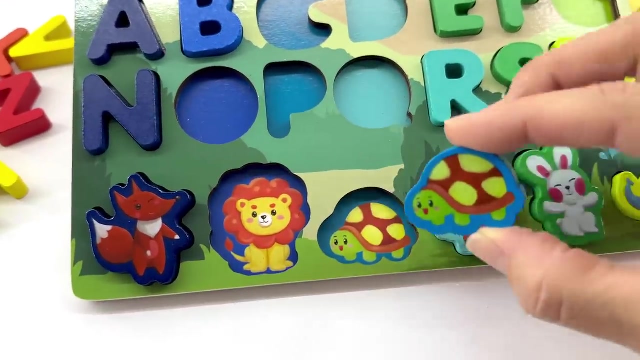 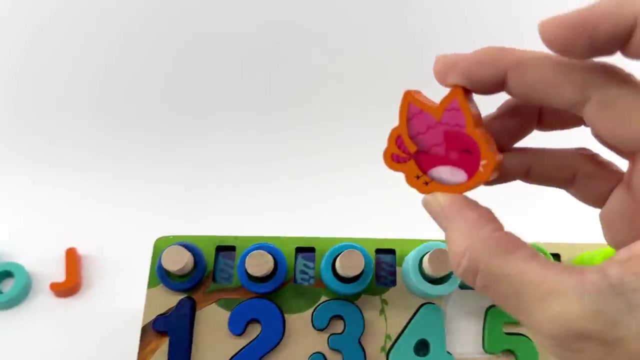 That we can choose from. Hmm, What about this one? Do you know what animal that is? Right, It's a turtle. Turtle starts with the letter T, T, T, T, turtle. So let's see if we're right. Yes, that's where the turtle goes. Let's do another one. What about this one? What is that? Right? It's a bird Bird starts with B, B. 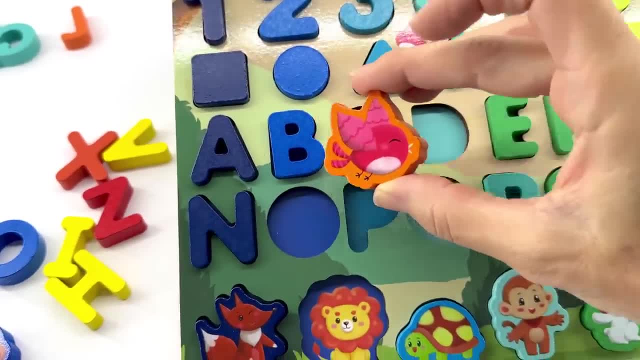 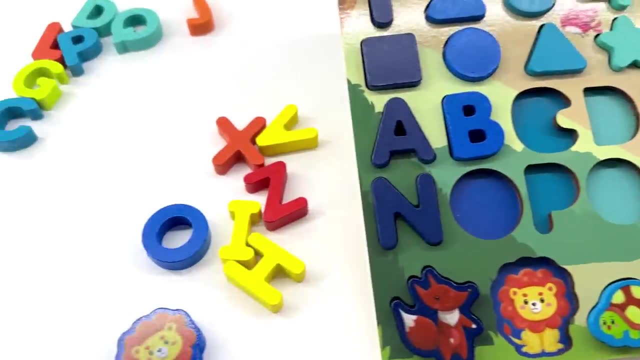 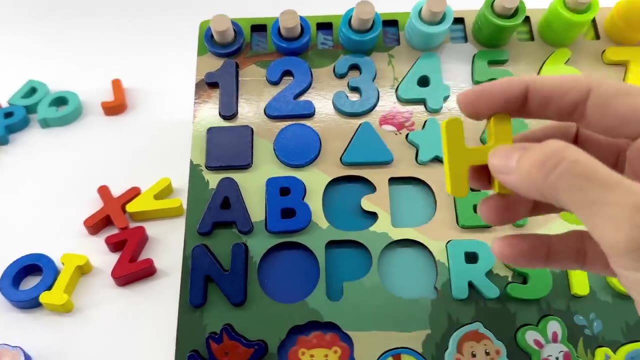 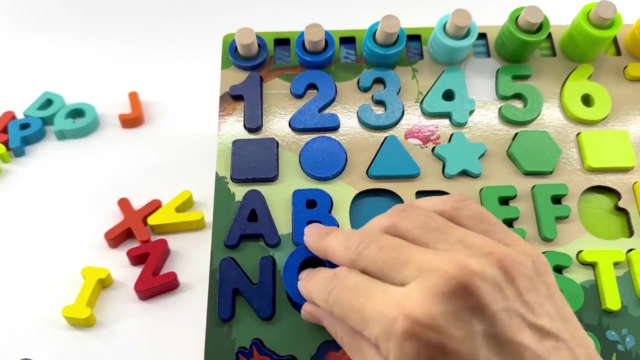 The letter B. There's the letter B, And where do we put our bird Right here? Great job, Let's do some more letters. How about the letter H? And that one is yellow, So let's put that right there. And how about the letter O? And that's blue. It goes after the letter N And now the letter C, And that's blue. 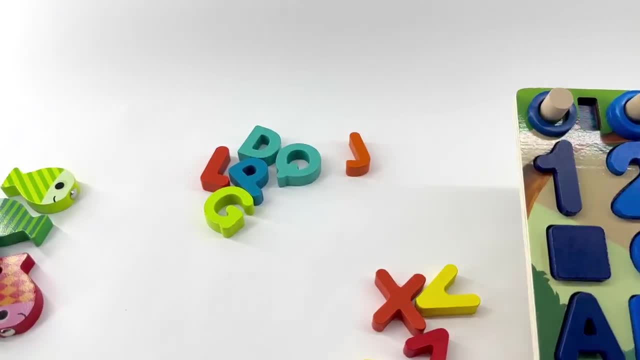 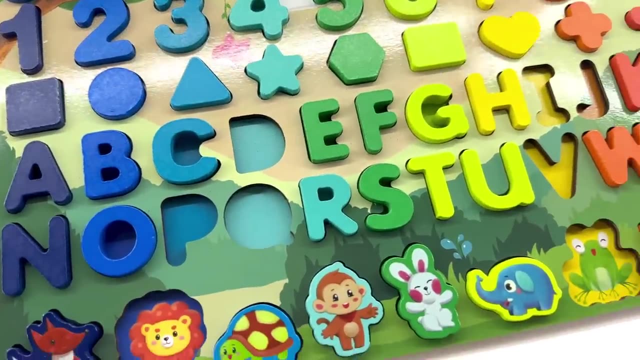 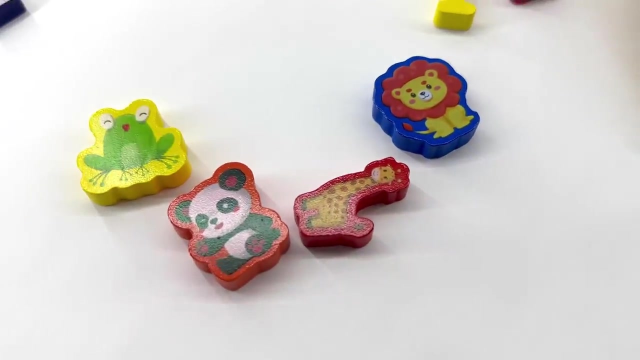 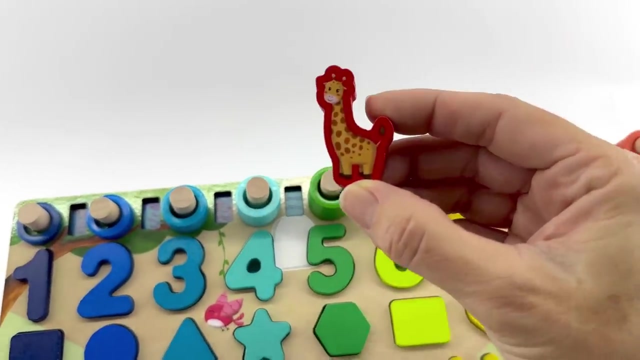 Also. And how about the letter G? That one's green G. Now we're just missing a few. Wait a second. I think I see an animal that starts with the letter G. Do you see an animal that starts with the letter G? Right, Giraffe, G, G, Giraffe. That's right, And let's see where it goes Right here. 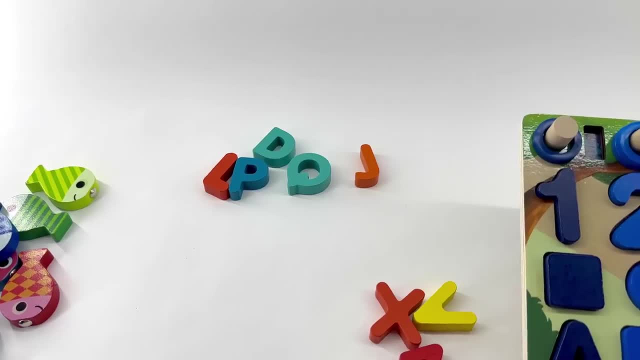 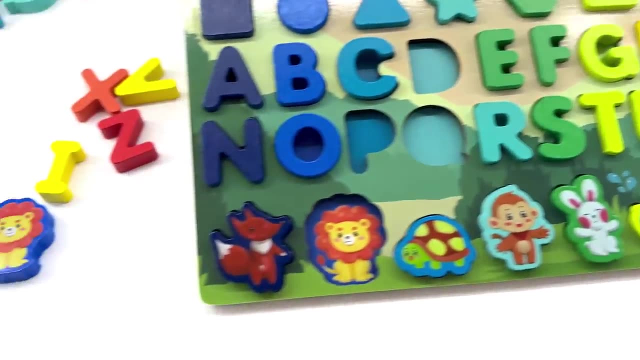 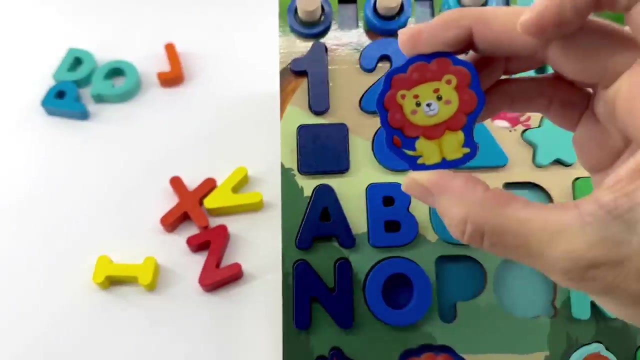 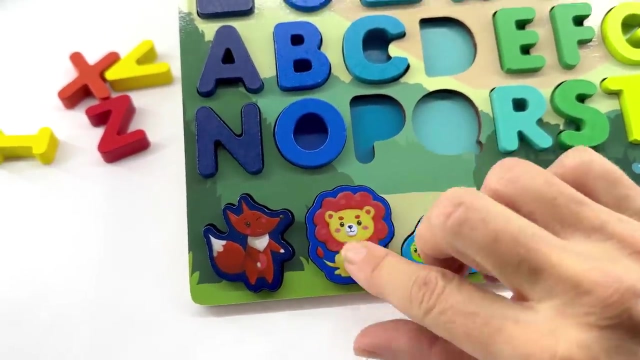 Okay, Great, Let's do this one. The letter L, And it's orange. I think I see another animal that starts with the letter L. Which one of these starts with the letter L? Yes, it's a lion. Can you roar like a lion? Roar Right, And here it goes to its home. Here's the letter I: It's yellow. 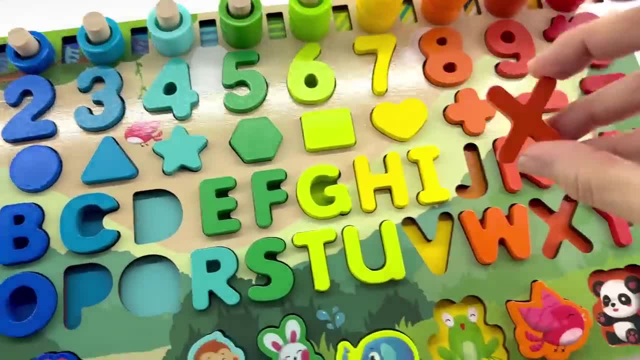 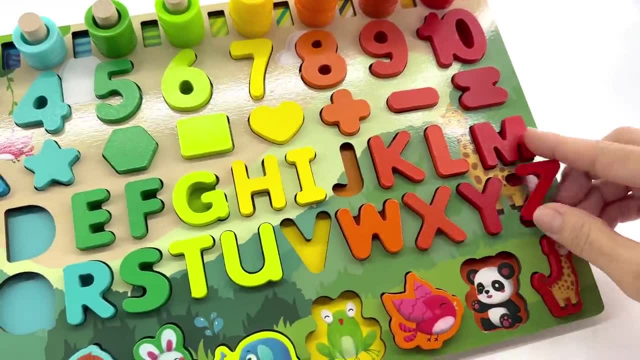 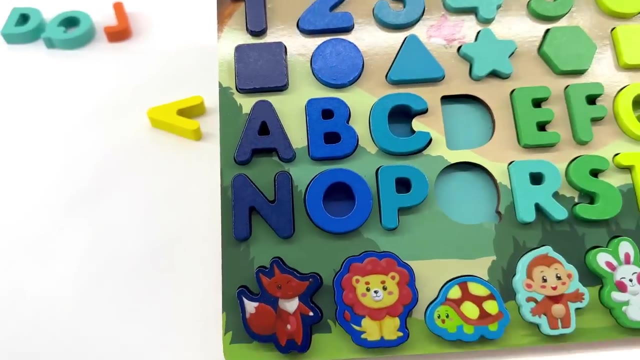 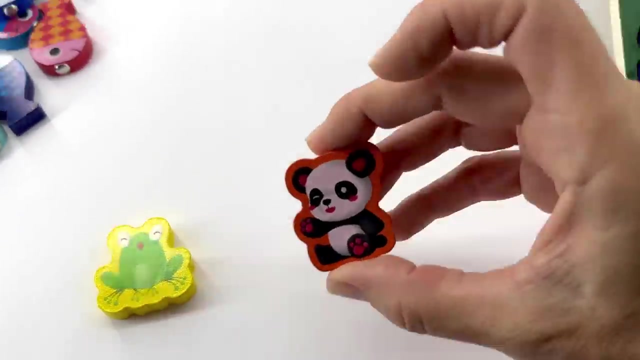 Here's the letter X, And it's orange. The letter Z Sounds like zzz And it's red, And here we have the letter P And this one's blue. It goes right there. I think I saw an animal that starts with the P. Which one of these animals starts with P? Right, It's panda. Panda starts with P. Let's put that one right there. 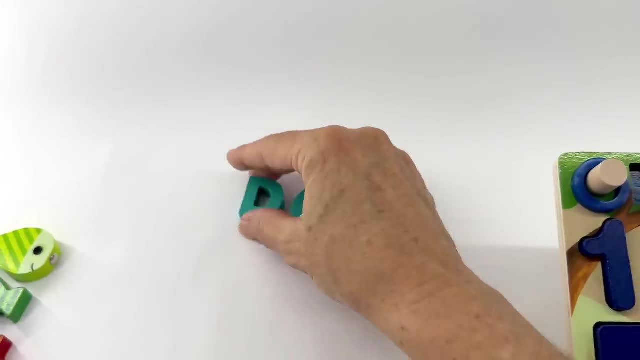 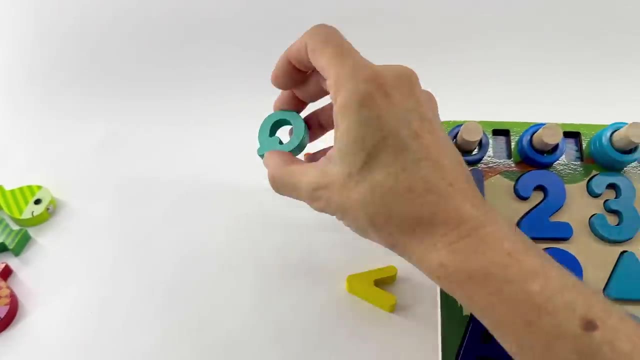 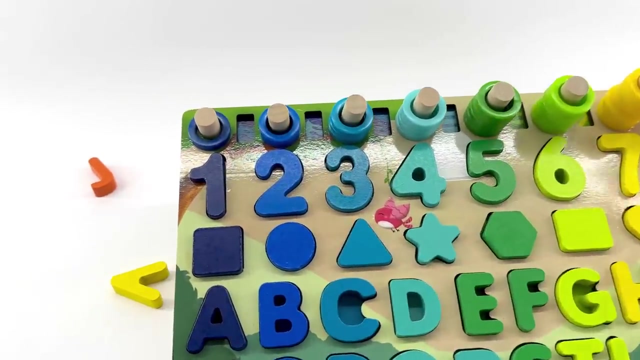 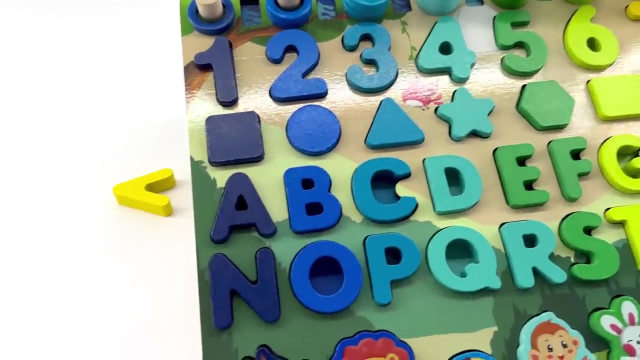 And let's finish our letters. We're almost done. D goes right there, Just like the dog, And Q. Do you know a bird that starts with the letter Q? Quail, Right, Whoops, Let's put that right there. And how about the letter J? Let's put that there. That one's orange. And our last one, It's the letter V, And it's yellow. 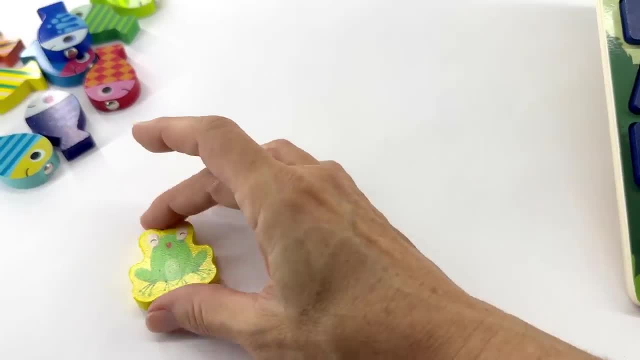 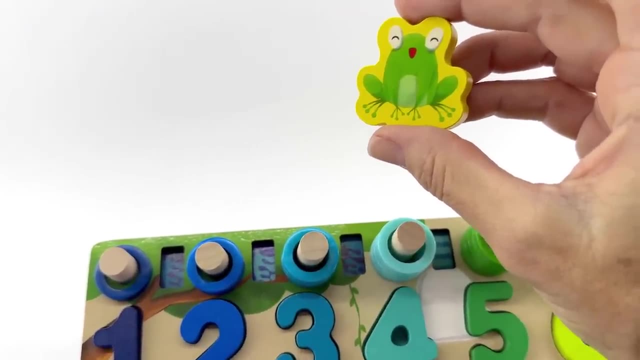 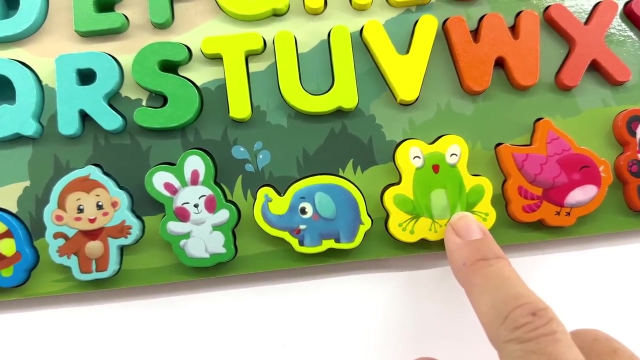 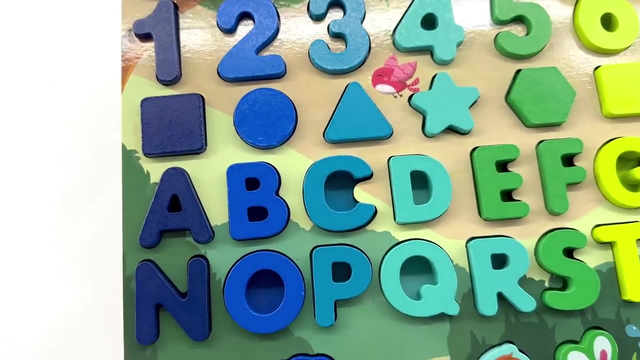 And let's put that right there. Hey, we still have one animal left. This is a frog. Frog starts with the letter F, F, Frog. Let's put it in its home. Right there. Do you know what a frog sounds like? Ribbit? Right, Let's say our alphabet together before we find all of our fish that need to come in here. Okay, say it with me. 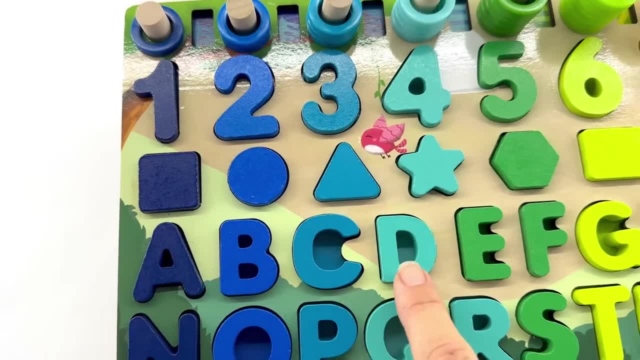 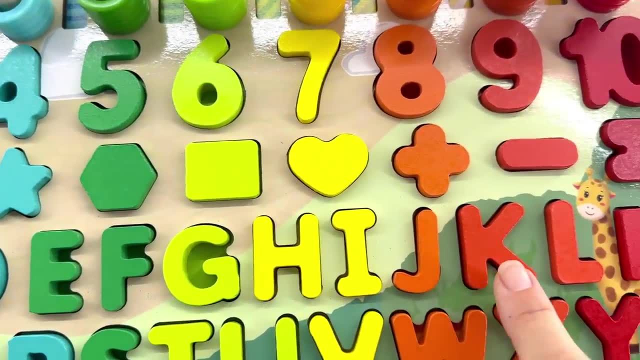 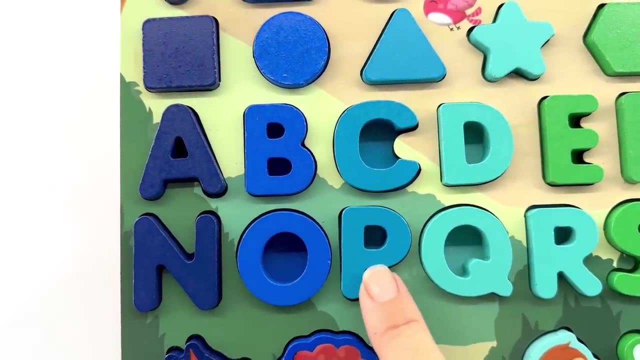 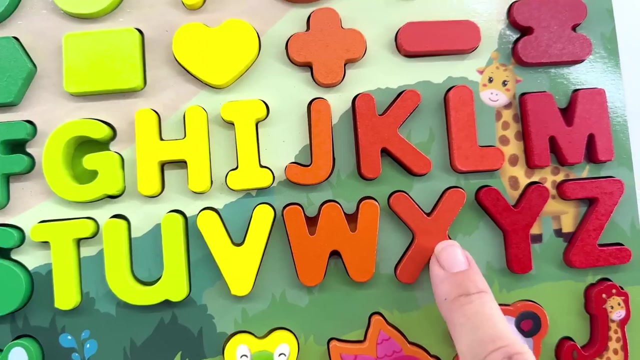 A, B, C, D, E, F, G, H, I, J, K, L M. Come back down here. N O P, Q, R, S, T, U, V, W, X. 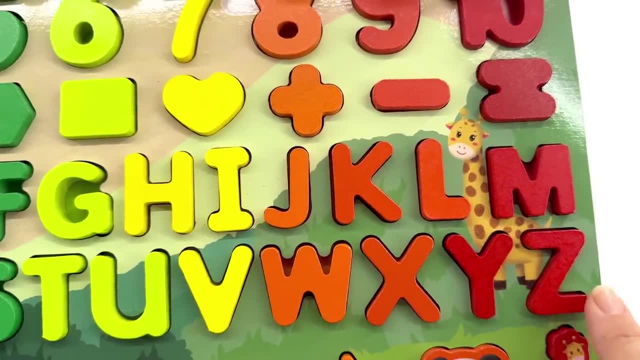 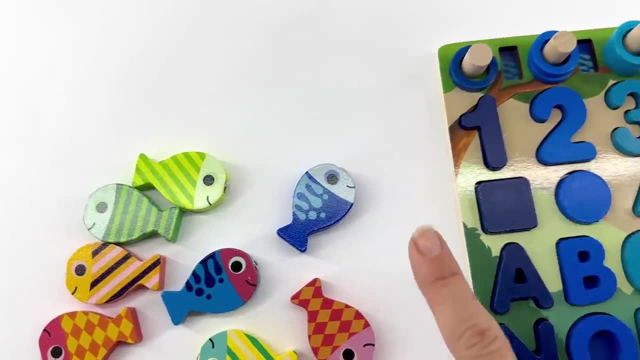 Y, And what's our last one? Z, Right, Great job. Now for the last part of our game. We need to find the fish that matches the color. But we can't just pick it up with our hand. We have to try to get it. 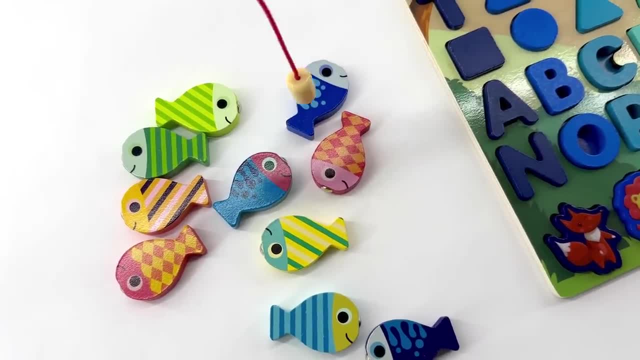 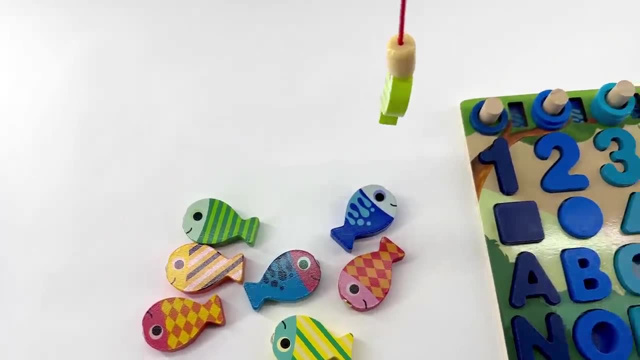 with this fishing pole. Do you think we can do it? I think we can. Which one should we try to get first? How about that one? Is it going to get it? Yes, it did. This one is green. Okay, let's try. 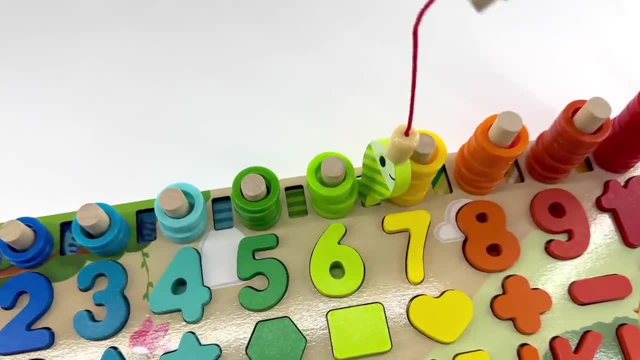 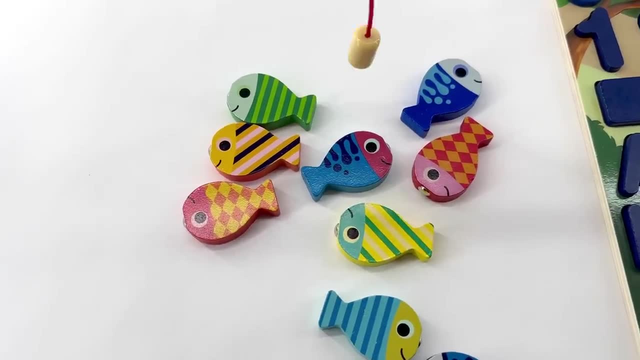 to put it here in our green spot. We did it, And now the green fish is in his home. Which one should we do next? How about a blue one? Let's see, Are you going to get it? Yes, we got it. 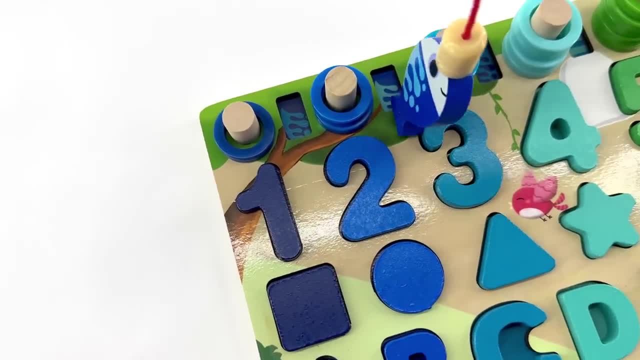 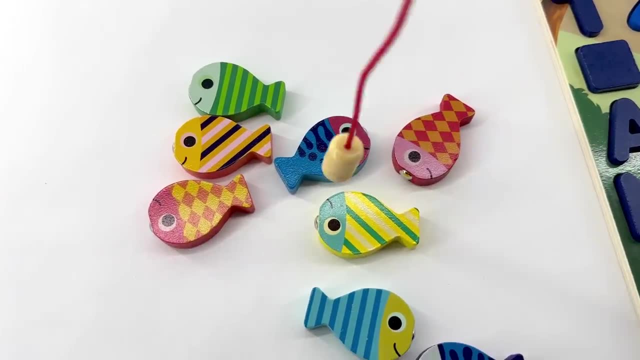 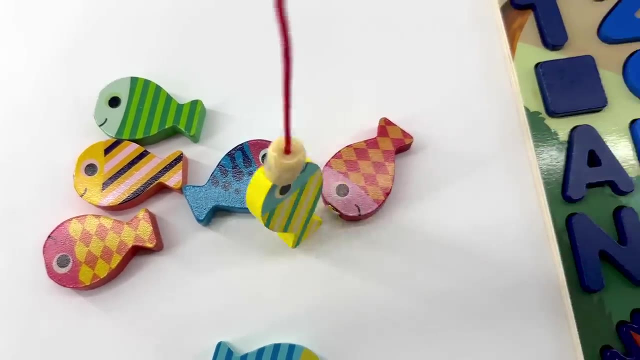 And now we're going to put it in the blue home. How about right there? Good job, Why don't we try this one? Hmm, You got it, Keep trying. Yes, we got it. This one looks yellow Okay. 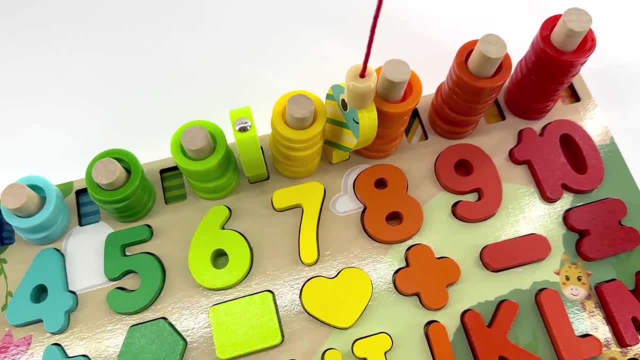 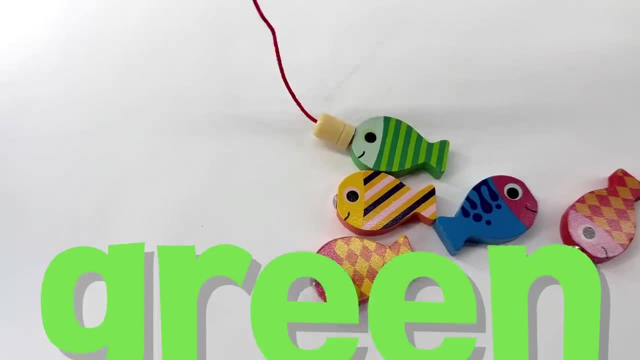 Let's try to put it here in the yellow spot, The yellow home, You did it again. You're doing great. And now how about the green one? Wow, that was fast. You're getting better and better. The green fish.